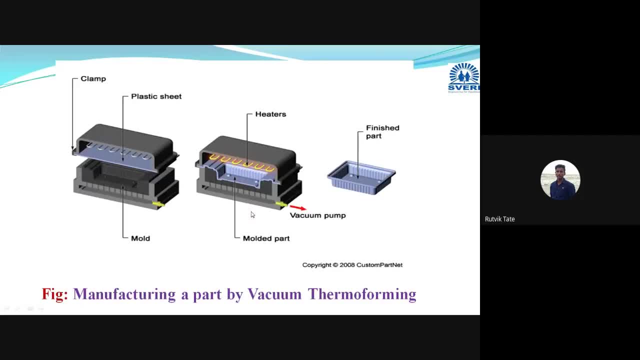 Okay, good afternoon all. Now I will welcome you all for this today's session. In this today's session we are going to deal with the concept of a thermoforming process, how the thermoforming process is performed on the plastic materials. Then it's a basic. 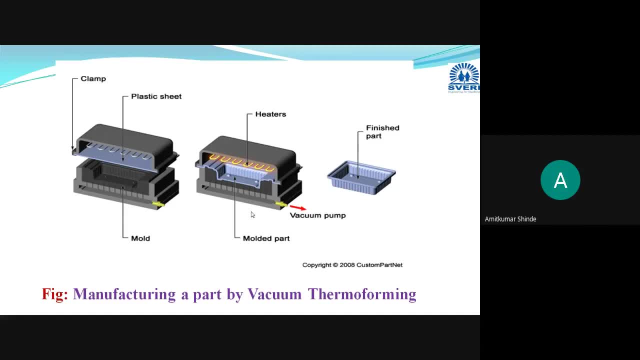 working principle in that we are going to study. It's a basic working principle, Then it's a different types. according to the some change of the mediums, some different types are there. Then after that we will discuss related to its basic advantages, disadvantages. 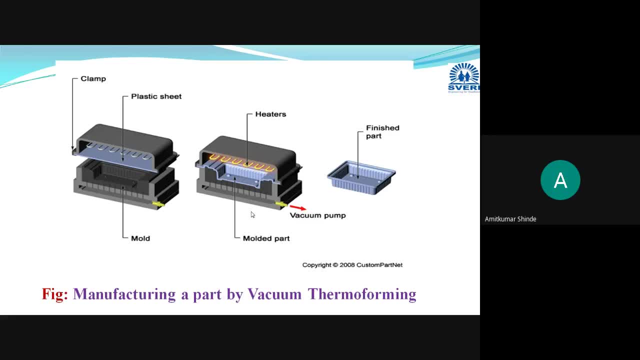 and some applications One by one. we will discuss that And after completing this concept of thermoforming we will move towards some. I have not discussed the MCQ questions in the lecture with the answers. I will discuss it And after that we can also try to attempt. 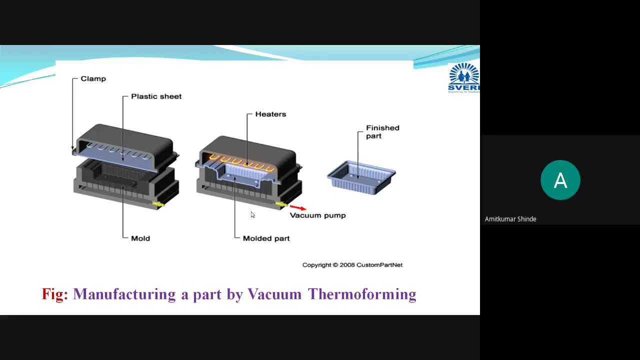 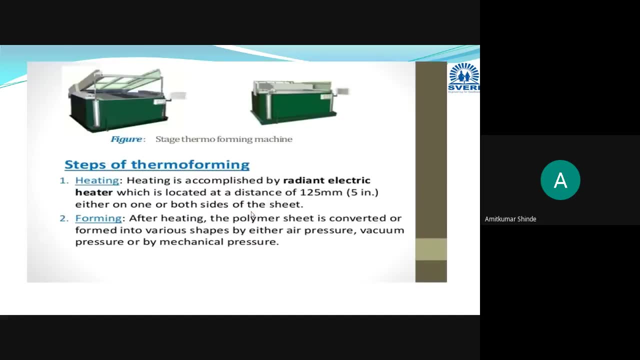 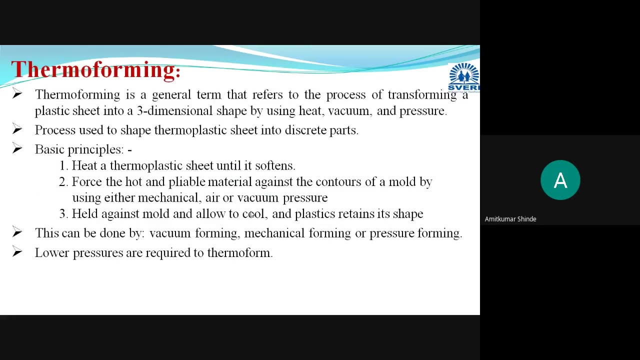 that whichever test I have shared, please solve that test also. Okay, I will start this session now. In this we will see the concept of thermoforming. Okay, Now, first we should know what is the meaning of thermoforming. Okay, Now, in this thermoforming, what we 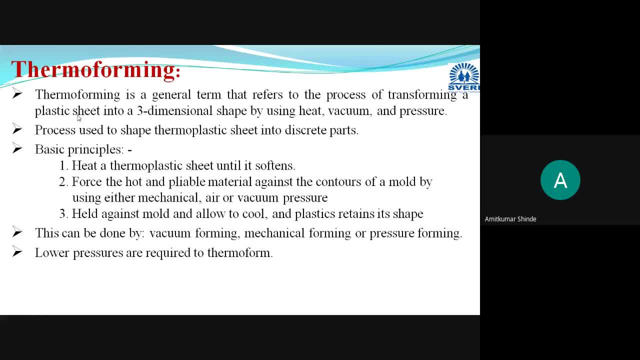 are going to do whichever sheet, whichever plastic sheet we have obtained at the end of calendaring operation: Okay, To that sheet, plastic sheet, we are going to give the desired three dimensional shape. Okay, And for doing this, to give the desired shape and size. to. 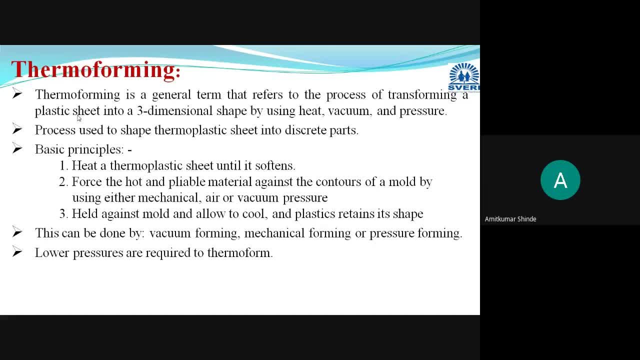 that particular available plastic sheet. we are going to use different measurements. mediums- okay, we are going to use vacuum, medium and pressure, medium, medium. or with the help of vacuum, with the help of pressure and with the help of heat, we are going to change the shape. 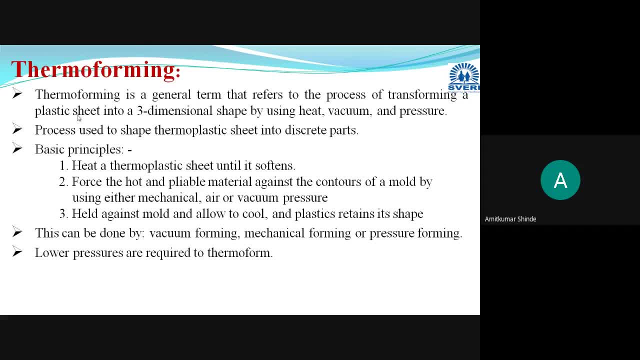 of that plastic material and, depending on that, we are having some different types for the thermoforming of the plastic material. okay, now, before going in the brief discussion related to its classification, first, what is the meaning of the thermoforming? thermoforming is nothing but, in simple words, to 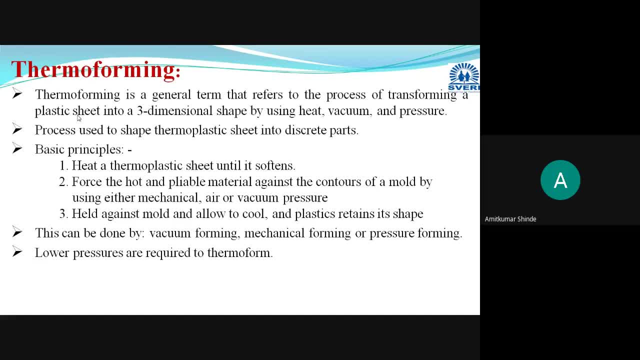 give the three-dimensional shape as per a requirement, with the help of heat, vacuum and pressure to the available plastic sheet. okay, that is termed as the thermoform: whichever plastic sheet is available to that plastic sheet is available to the available plastic sheet sheet. we are going to give the desired shape 3d shape. okay, now in this thermoforming, the basic. 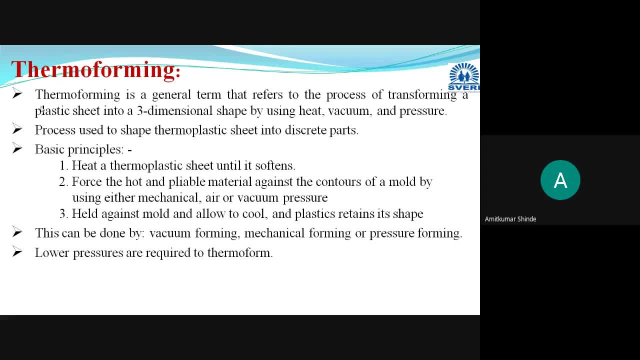 steps involved in that process, the first stage, or here i have explained the basic principles before that we are going to study the basic principle first. you should understand that this process can be performed only on the thermoplastic materials. okay, here we cannot go for the thermosetting material. okay, as in the previous sessions we have already discussed. 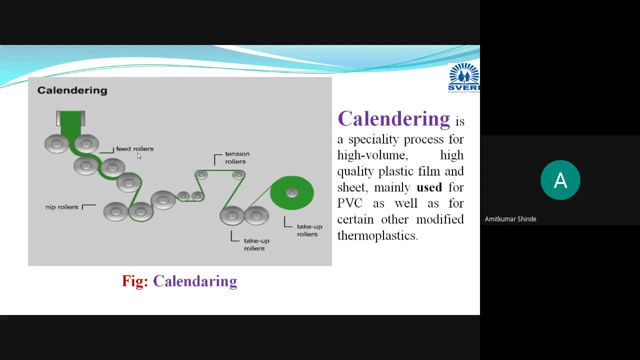 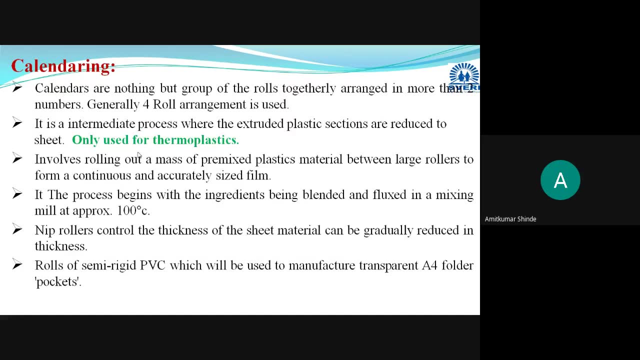 i will just summarize it. what is the meaning of calendaring? okay, whichever output you are getting at the end of this calendaring process. what is the calendaring? okay, calendaring is nothing, but with the help of this rolls- okay, different types of the rolls, whichever raw. 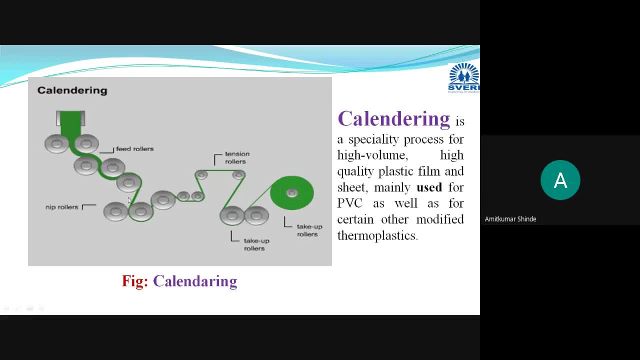 material is available- plastic raw material. that plastic raw material is converted into thin film with the help of, by applying the pressure, by or using the rollers- okay, different rollers may be there- and at the end we will end up with the thin plastic sheet of that material. and this process we 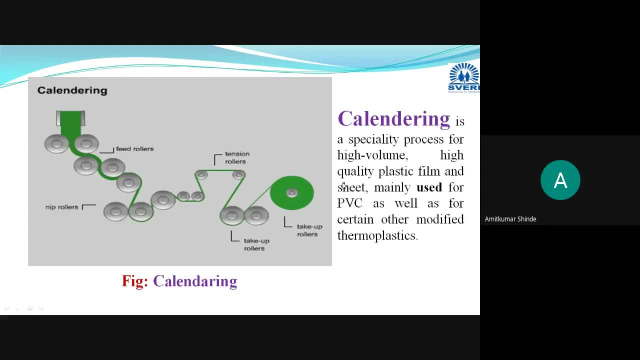 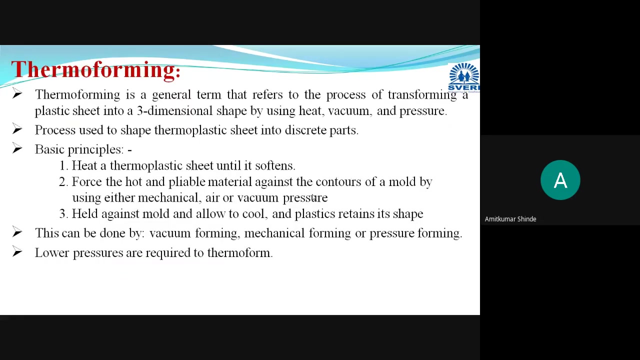 can conduct on the thermoplastic materials like pvc, or you can say that the polyethylene, etc. okay, now, after getting this fine sheet- okay, thin, thin sheet- is obtained. now we are towards. So what i am doing here is for one kind of earth 선생 that will give shape to that sheet. 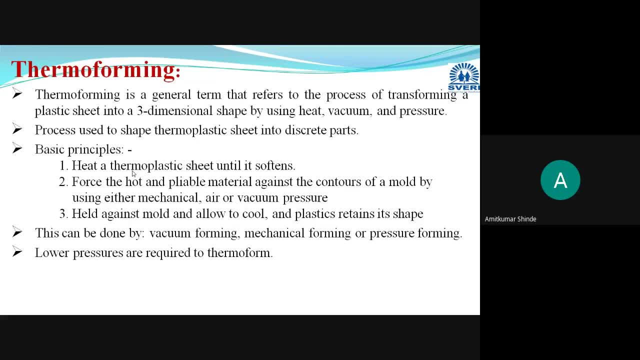 then for that I have to apply some pressure on it. some heat and some pressure to give it a desired shape and size. that process will be termed as the thermoforming process準備ję أطول بال ثریور essay أطول أformation. 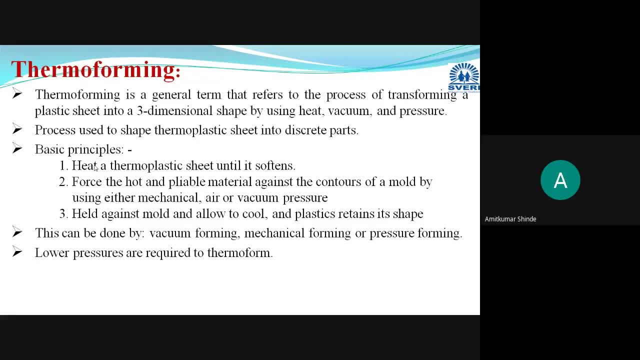 we are going to heat it until it softens. okay, we have to make it soft for the further processing. that is the first step: heating the thermoplastic sheet until it softens. then, after heating it, we are going to apply the force. okay, whichever softened material is there heated, you can say: 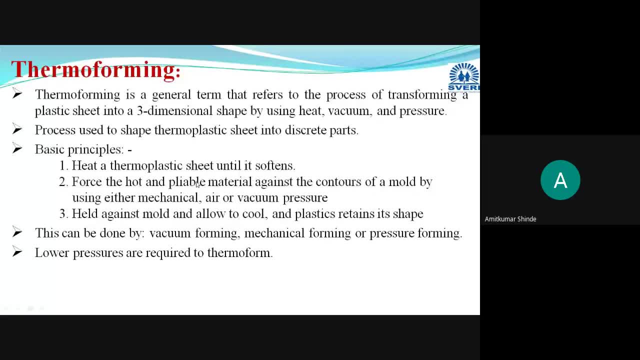 that that is hot and pliable material. hot and pliable means pliable material means you can perform the bending or shaping operation on that material. it is termed as pliable. okay, now on that hot. in the first stage we are going to heat the thermoplastic sheet until it softens. then, now that 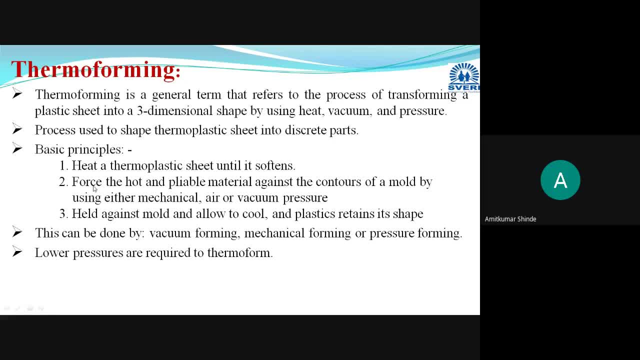 sheet is hot and pliable. now we can apply the force. okay, now this force can be applied by using, like you can go for mechanical mechanism, then you can go for air pressure or vacuum pressure. also, in the second step we are going to apply the force and in the third step, it is allowed to cool. 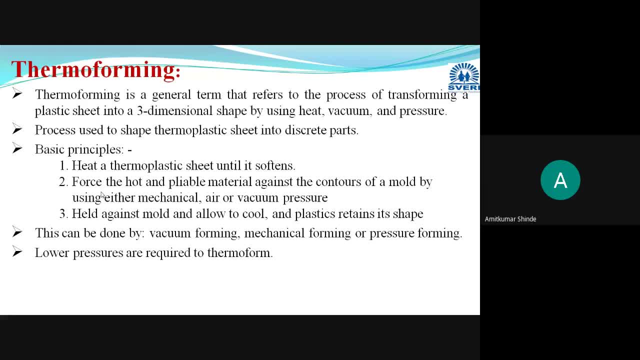 and after that cooling, that material will acquire the desired shape and size and we will end up with the final product. okay, in this way, the thermoforming process consists of three stages: first is the then applying the force, and third is the cooling process. okay, just you have to provide some. 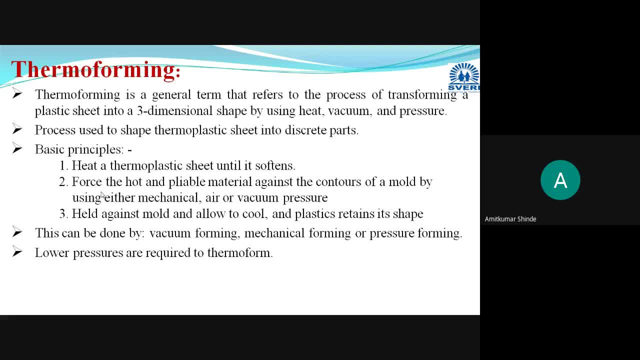 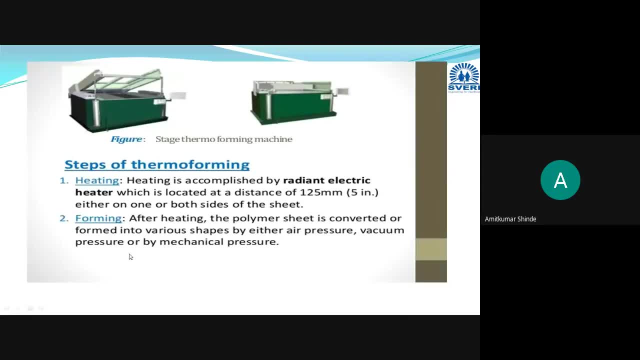 cooling time so that it will acquire the desired shape and size. okay, now this basic stages are explained here only. okay, generally this forming consists of. you can say that these three stages i have summarized in the two steps only. the first stage is the heating and second stage is forming. 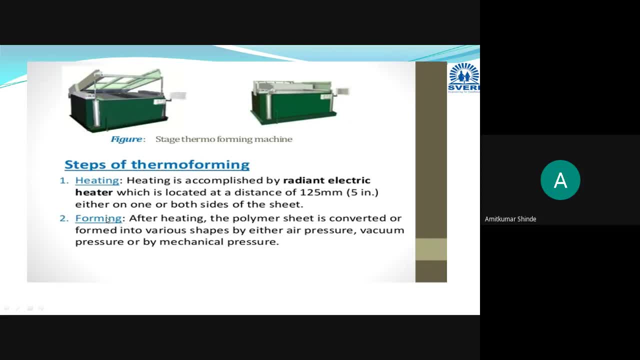 okay, together here the applying. i can say that the whichever pressure we are applying here or force we are applying- force plus cooling- that is termed as forming here. in this way in some books they have explained it in the two stages: only in this forming stage force will be applied and it is 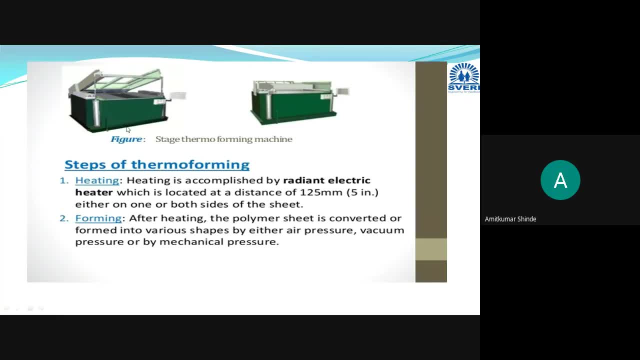 allowed to cool to get the final product. okay, now this is the thermoforming machines, different thermoforming machines which we are using in the practical life here and the first stage, heating is done with the help of a radiant electrical heaters. okay, and from one side, or both sides, and we are going to do the heating depending on our need, okay. and 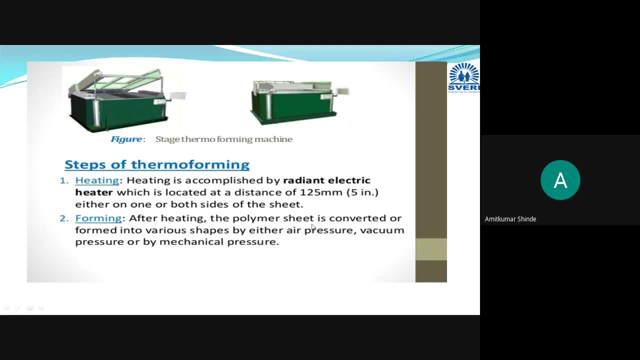 after heating and the whichever plastic or polymer material sheet is there, it is converted or formed into various shapes, either by air pressure, vacuum pressure or by mechanical pressure, followed by the cooling to get the desired product. okay, so this is the basics of the thermoforming process. now, 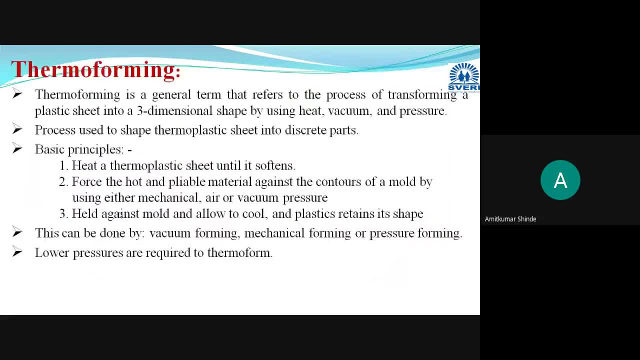 the next is the types of the thermoforming process. okay, here already i have explained it- we can apply the force with the help of a vacuum medium. you can go for okay, the medium. you can go for pressure medium or directly. you can apply the pressure also. you need some help of home press layer. you can apply the pressure also, or with 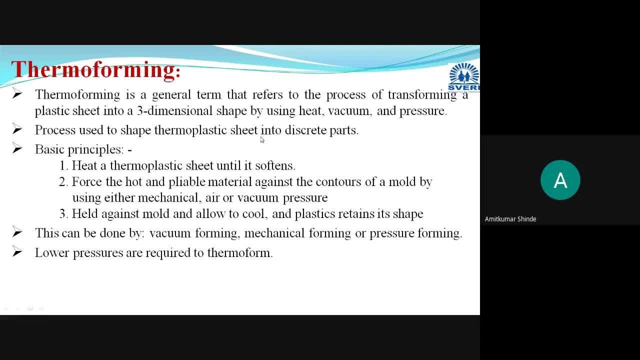 the help of some mechanical tools, we can apply the pressure now. in this way, this thermoforming is classified in three times: vacuum for thermoforming, mechanical thermoforming and pressure thermoforming. okay, one by one, we will discuss these three thermoforming processes now. okay, if you are having any, 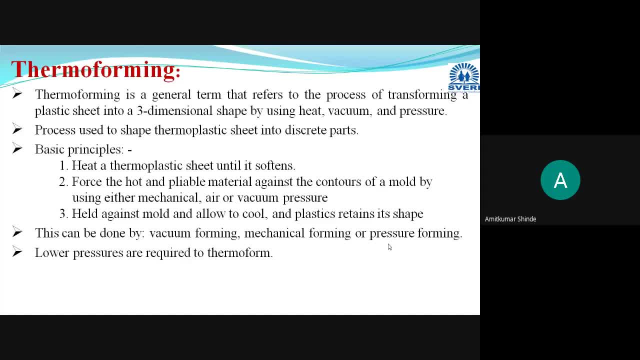 doubt related to the basic concept of this thermoforming. you can put that in the chat box. I will wait for one minute here. after that I will move towards the different types of the thermoforming. first we will go for pressure thermoforming. okay, if you are having any doubt, you can ask me here or directly. 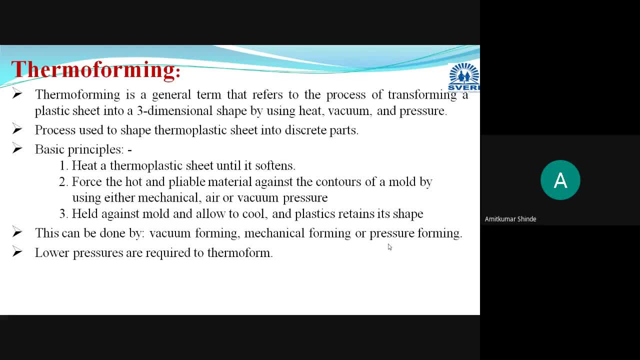 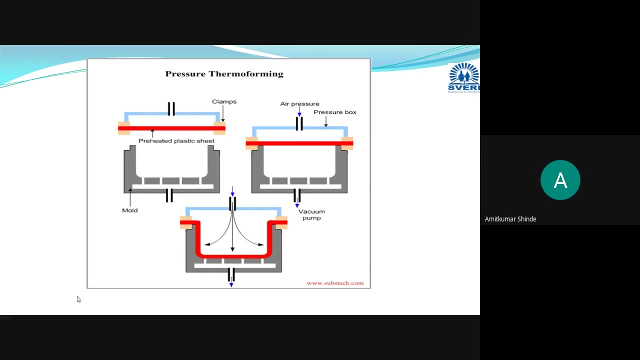 unmute yourself and you can ask me doubts. you can put that in the chat box. and another basic thing: you have to take into consideration that here in this thermoforming processes, some lower pressures are required. we are not going to use the high pressure values. okay, if you are having any doubts, you can put that in the chat box. okay, thermoforming. 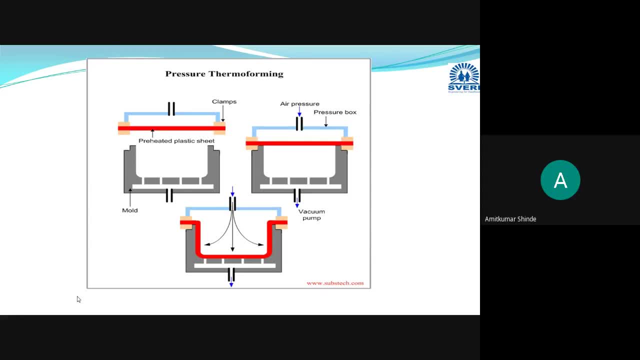 here, whichever sheet is plastic sheet is obtained at the end of our by performing the calendaring operation on that plastic sheet, we are going to apply the heat and force to convert it into the desired sheet. we are going to apply the heat and force to convert it into the desired sheet. 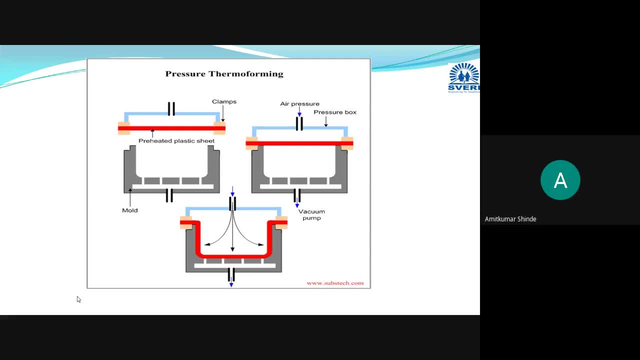 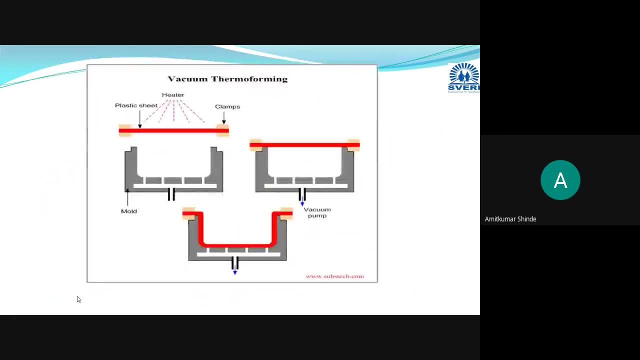 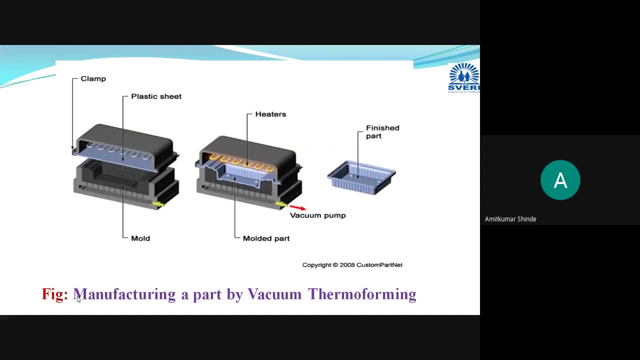 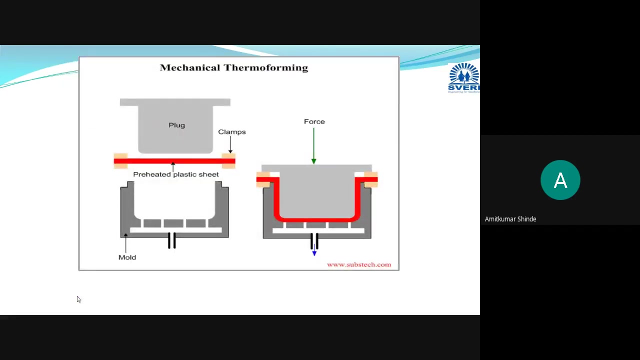 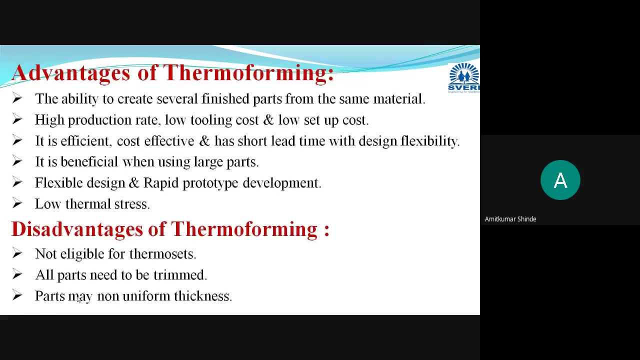 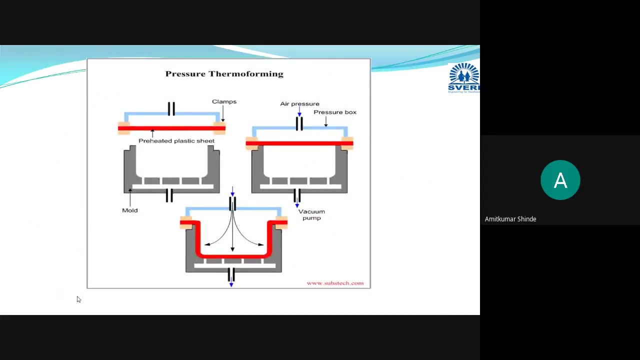 the 3d shape. this process is termed as the thermoforming. okay, now we will move towards the types of the thermoforming process. the first type is the pressure thermoforming. okay, here, with the help of these diagrams, I will explain this pressure thermoforming. how the actual pressure thermoforming. 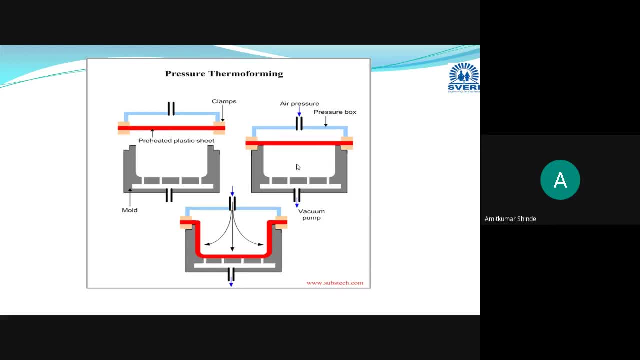 processes are completed here now. I am going to explain how the actual pressure thermoforming processes are completed here now. I- this red color is your preheated plastic sheet. okay, please try to concentrate on the cursor. okay, I will show the cursor. please try to concentrate there. according to that, you will understand the stages. this first: 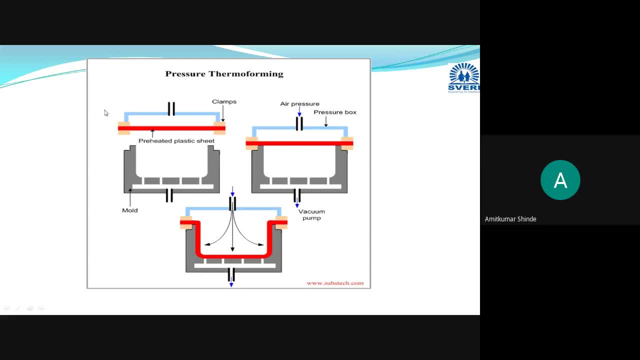 this left corner diagram. left top corner diagram. this indicates the first step. okay, here, whichever plastic sheet is obtained at the end of calendar hi-gov, that plastic sheet is collected and it is preheated, or you can say that directly. you can study that it is a heated, while the term preheated is used. 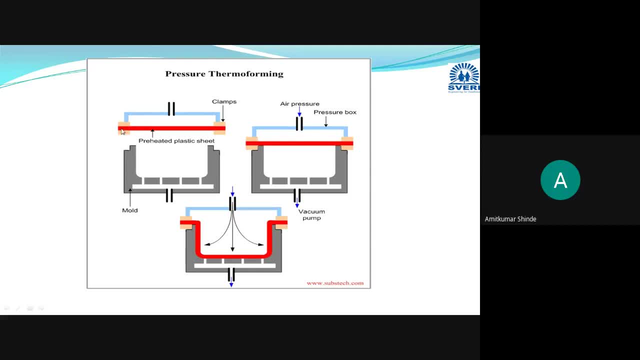 to give a fully performing or applying that force. it is heated. that's why it is here. we are going to perform the electrical heating. okay, electrical heating is done in the on the stage and after the electrical heating. this is the first stage. electrical heating is done then in this second stage, this here, it is placed on the mold. okay, whatever shape you want to give. 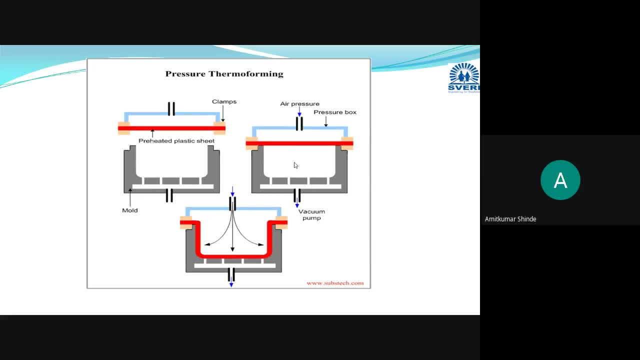 that particular sheet. you want that particular sheet in that desired 3d shape. according to that, you have to give the design to the mold. okay, on that mold, that material is placed, or you are heated. heated plastic sheet is placed and with the suitable arrangement. okay with this suitable. 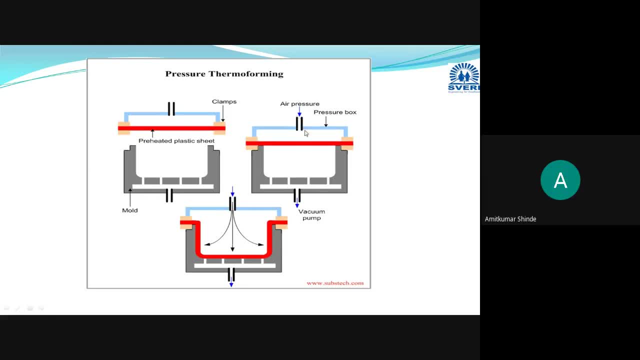 arrangement from the top surface. okay, there we are going to apply the air pressure. okay, here we are going to apply the air pressure. now, due to the air pressure, what will happen? this air will flow. okay, it will apply the force. and due to he heating process and this thermoplastic material, 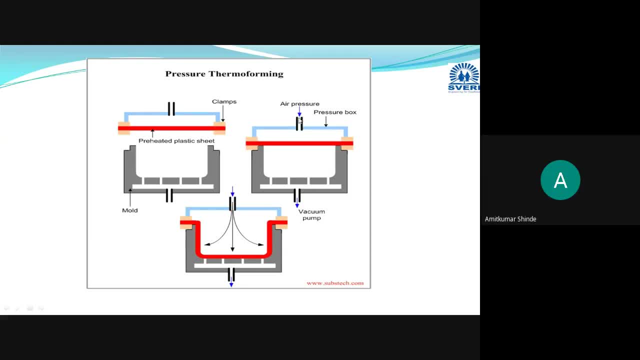 has become soft in nature and due to this force, it will means due to that force. what will happen? whichever material is there, or that sheet is there, it get placed against the mold wall. okay, this is the mold wall. this is the mold wall. due to this pressure, this sheet will get placed against the 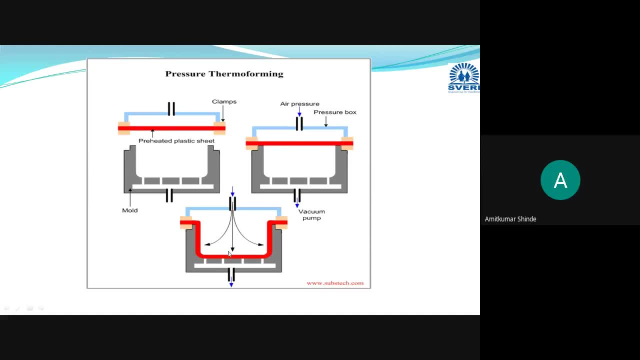 mold wall. okay, it will get placed against the mold wall and here we are allowing it to cool and after sufficient time, and uh, here at the bottom side, when vacuum pump arrangement is also there, uh, you know, with the help of this vacuum pump the extra air is taken out. okay, and this extra air is taken out. 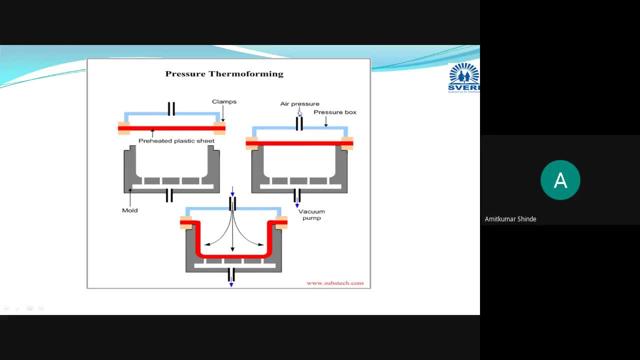 before applying the pressure. okay, before applying that pressure from the top surface, this, whichever air is there in that mold mold cavity, that air is taken out and after that the pressure is applied. and what will happen? due to the applied pressure, that sheet will get forced against the mold cavity walls and it will acquire 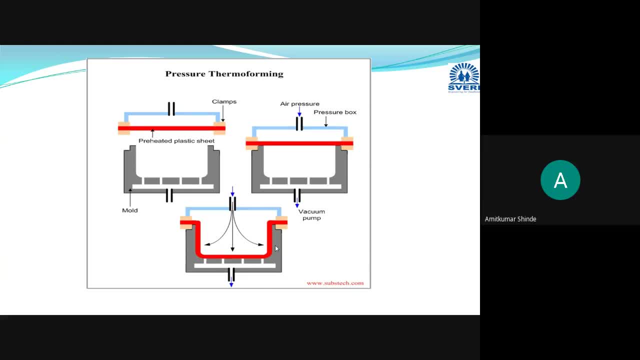 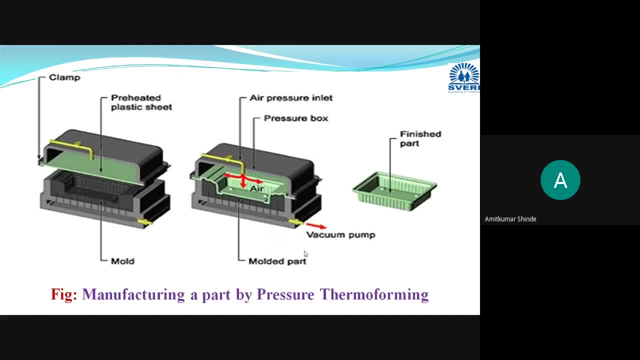 the desired shape and size and some time is given to given for the cooling, and we will end up with the product, final product with the desired shape and size. okay, this same operation. okay, I have explained with the help of one- uh, you can say that one- practical example. okay, this is. 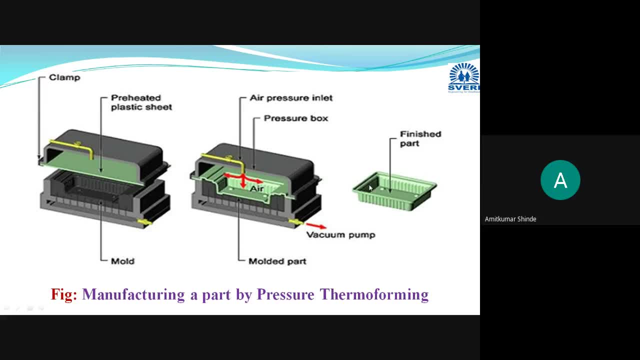 the practical example. this is your final product. okay, please first check your final product. this is the final product. you can say that one dish or one plate is there. this can be manufactured with the help of pressure thermoforming. now, this is the clamp arrangement. okay, this is the clamp arrangement. 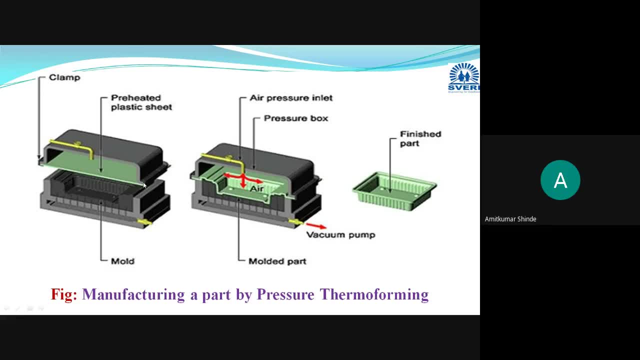 initially, this uh plastic sheet is taken, plastic sheet is taken and now it is heated. okay, this sheet is heated with the help of electrical heating. then after that, here at the bottom side one vacuum pump is there and whichever air may be there, that air is removed from the this mold cavity or mold box, any 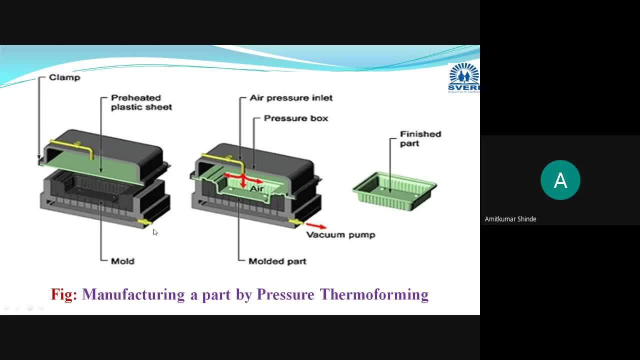 type of air may present, it is eliminated with the help of this vacuum pump. now, in this second stage: okay, we are going to place this sheet on this mold box, and from the top side, okay, pressure is a lot. pressure is applied by using some air pressure or compressed. 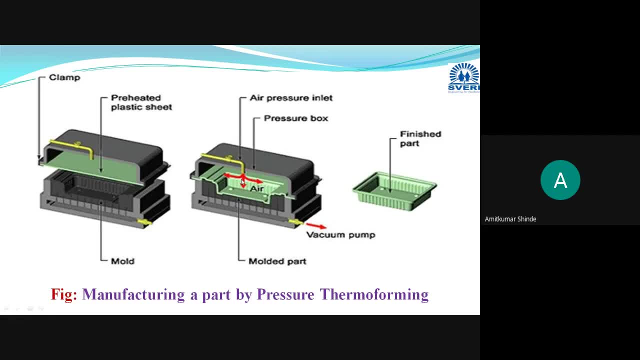 air is allowed to flow through that and in that mold box. so pressure. what will happen here? whichever, that mold cavity is having, that shape is acquired by that sheet as, due to the heat, it has become softer in nature and due to that pressure it will acquire the required shape and size and, after some providing some time for cooling, you will end. 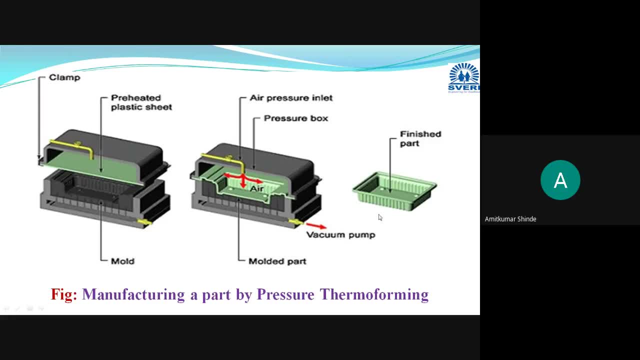 up with this final product. this is the finished product. one dish is manufactured, or one plate is manufactured. okay, this can be used for packing of the foods. okay, in the food industry, these kinds of the plates are used for packing the foods. this is the pressure- thermoforming- if you are having. 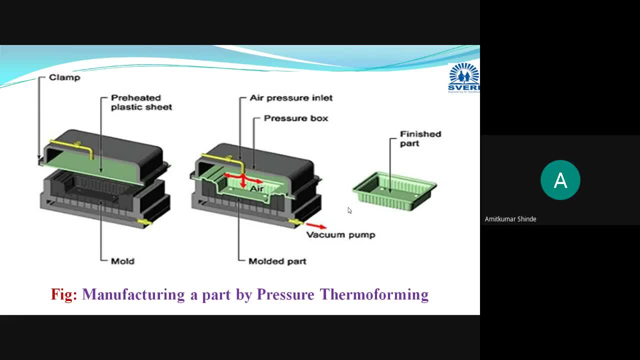 any doubt, you can ask me. i will wait for one minute here. after this, i will move towards the next type of the thermoforming. the concept is same in all three types, just we are going to change the mode of applying the force. okay, if you are not having any doubts, i will move towards the next type of thermoforming. this is the. 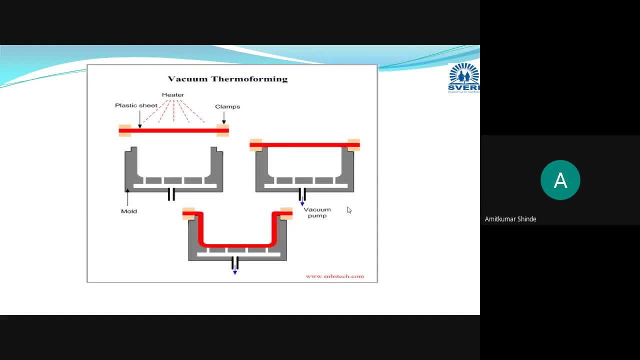 next type of the thermoforming: vacuum thermoforming. okay, these are the steps in all and this is the schematic arrangement for vacuum thermoforming. now, in the first stage, we are going to do the heating of the the thermoforming. so we are going to do the heating of the. 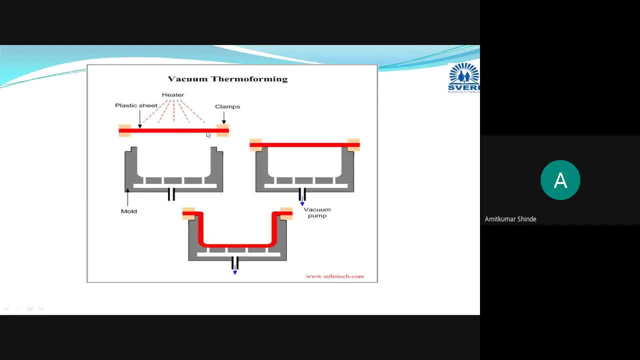 sheet. okay, now this sheet is obtained. plastic sheet is obtained by performing the calendaring operation on the raw material in that calendaring. we are going to apply that. with the help of rollers, we are going to convert that available raw material in the thin sheet and that thin 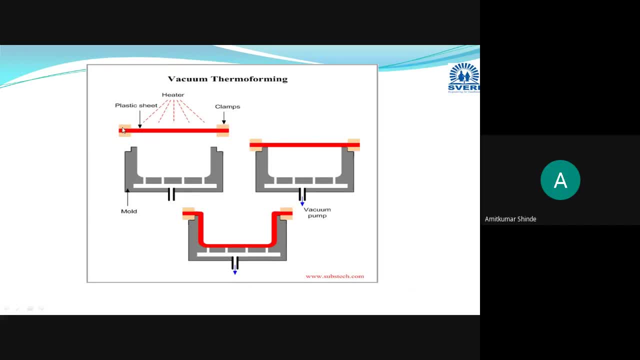 plastic sheet is. we are holding it with the help of some clamp or clamping arrangement and we are going to heat that sheet. okay, with the help of some heating system or heaters or electrical heaters, we are going to heat that sheet and after heating that, that sheet, that heated sheet, 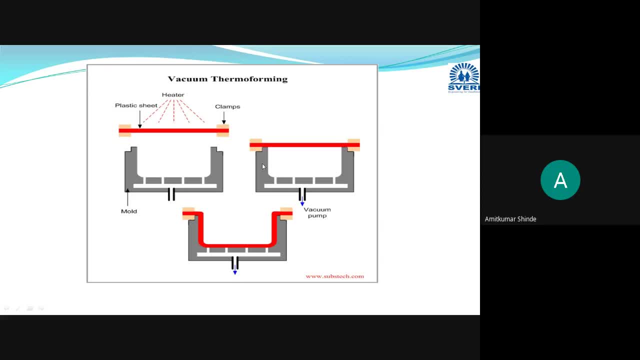 okay, that heated sheet is placed on the- uh, the mold cavity. okay, mold cavity or mold box, and that mold box or mold cavity, you have to provide whichever shape and size you want for your final product. that shape and size is provided here and it is placed on that clam. and now, 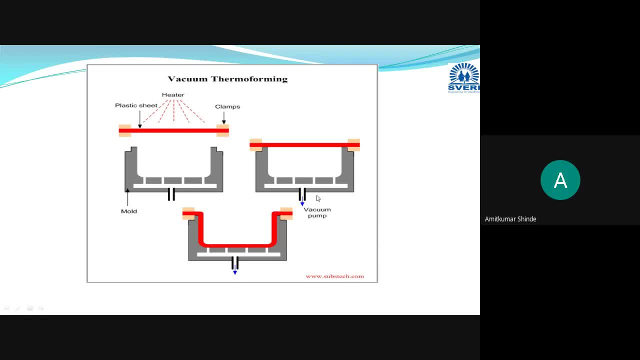 here. by attaching one vacuum pump, all air is taken out from this box. okay, all air with the help of vacuum pump. you can see that it is taken out from the vacuum box and, as this sheet is heated, it is soft in nature and, due to the pressure, 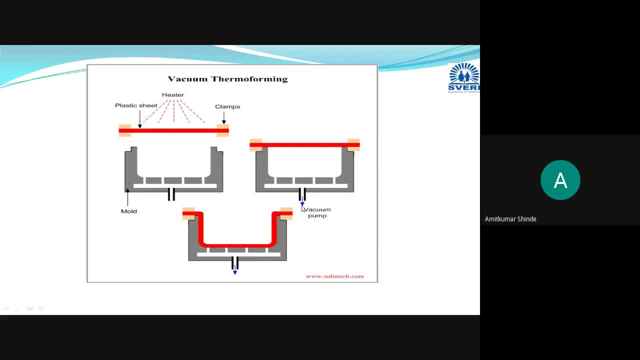 when you are taking the air out from this, from the bottom side with the help of vacuum pump, some okay, when force is created and due to that force, what will happen? and this thin sheet, it will get forced against this, whichever wall of this mold. okay, in this shape or in this way, it will get forced against the mold. 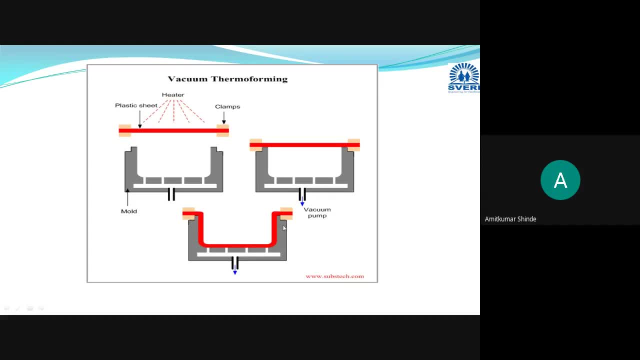 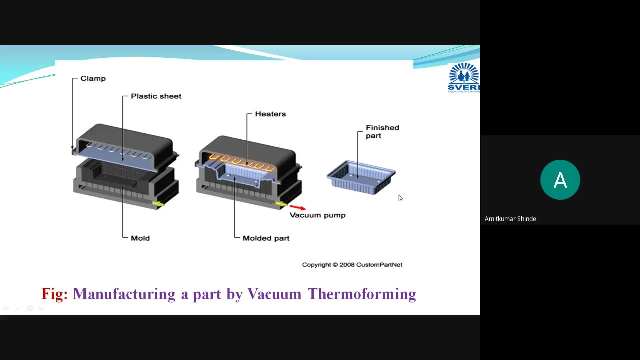 walls and, after sufficient cooling, you will end up with your final product. now, this same concept is a help. have collected one extra diagram, the same component. okay, whichever component, one box we have, packaging box we have manufactured here, or one plate or dish, you can say that in the initial stage, with the help of clamp arrangement, that 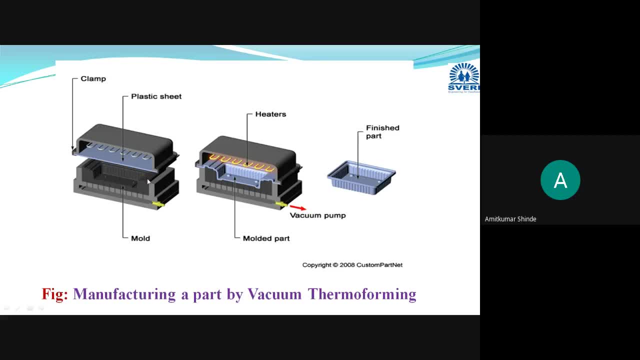 sheet is cold and it is heated. okay, it is heated here. you can see here, when heater, some heating arrangement, is provided with the help of these heaters, it is heated and in the second stage- this is the second stage- the air is taken out from that mold with the help. 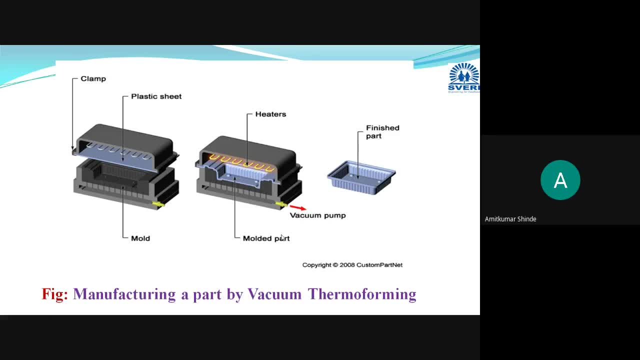 of a vacuum pump. with the help of a vacuum pump, air is taken out and you to this vacuum pump. this will get forced against the mold walls and it will acquire the desired shape and size and, after the sufficient cooling, that more box is released and we will end up with this final product, or this is the 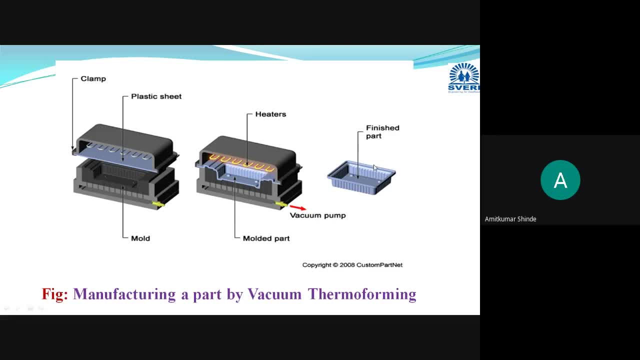 initially product to obtain at the end of this video, so that you get the result very soon of the vacuum thermoforming. okay, whichever force is required to give the desired shape and size that is, uh, applied with the help of that vacuum pump. that's why this process is termed as vacuum. 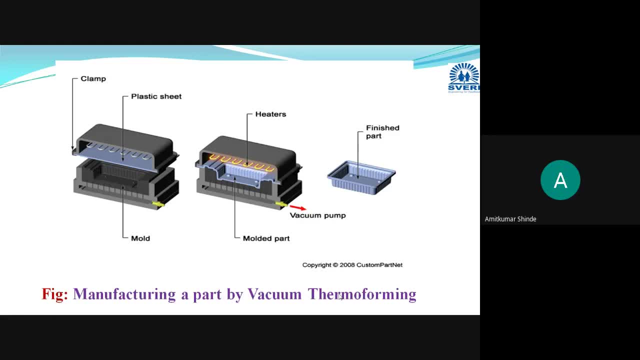 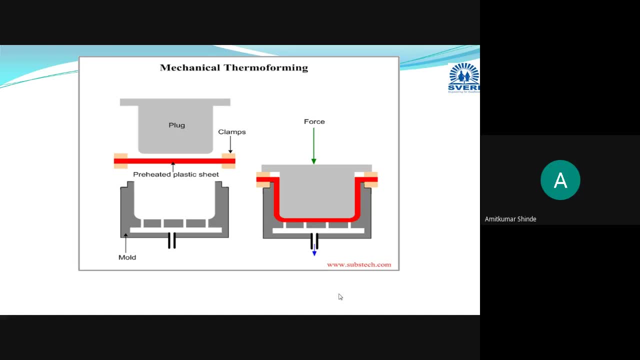 thermoforming. this is termed as vacuum thermoforming. then we will move towards. the next is the mechanical thermoforming. okay, if you are having any doubts, please ask me. so okay, then this is the last type of the thermoforming process: mechanical thermoforming. now, this mechanical for thermoforming very much similar to other two types. same stages will be there. 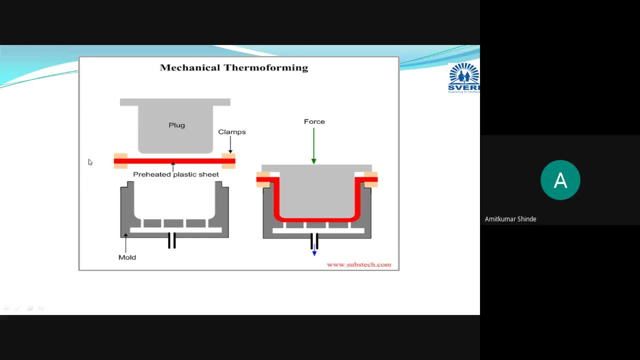 in the first stage, heating of that plastic sheet is done. in the second stage, force is applied, and in the third stage, after sufficient cooling, it is released from the mold box or that mold cavity to obtain the final product. now, here only the medium to apply the force. 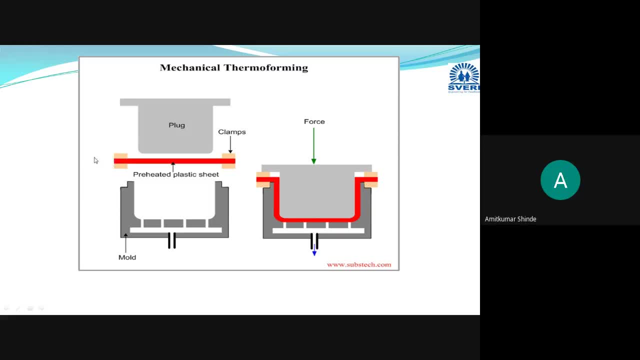 is different now. in the first stage, the plastic sheet is collected and with the help of clamping arrangement- it is you know, you can say that you can hold it and some heating is done on that sheet. heating is done on that sheet with the help of some heating system or heating heaters. different: 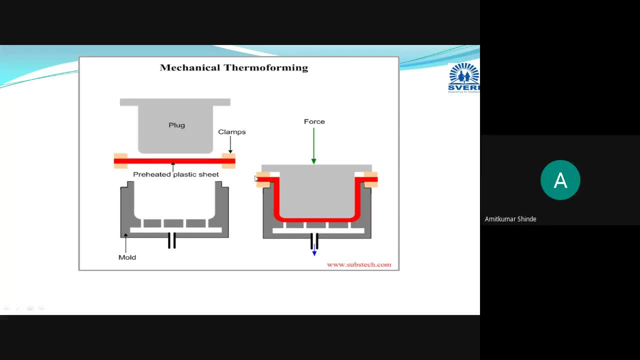 types of the heaters and, after heating it, it is placed on the mold and that mold cavity. you have to provide the desired shape and size which you want for your final product. then it is placed on that and with the help of one plunger, with the help of one plunger or a punch, in the second stage. 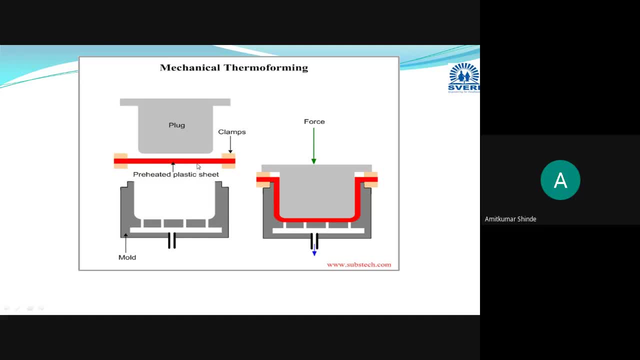 after heating the sheet and it is placed. it is placed on this mold and after that the force is applied with the help of that punch or plunger and due to that force, what will happen? due to the force it will move in, this force will be applied in downward direction and due to heat that sheet, 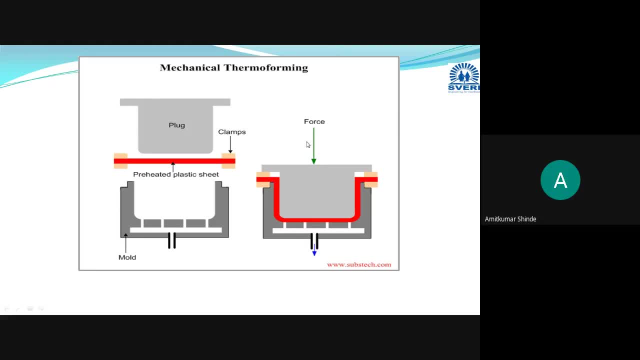 has become soft in nature and, due to the force applied with the help of this plunger, the material- plastic material- will get forced against the walls of the mold and it will acquire the shape of that mold cavity. okay, and at the end- or you have to provide some sufficient cooling time, after that you will end up. 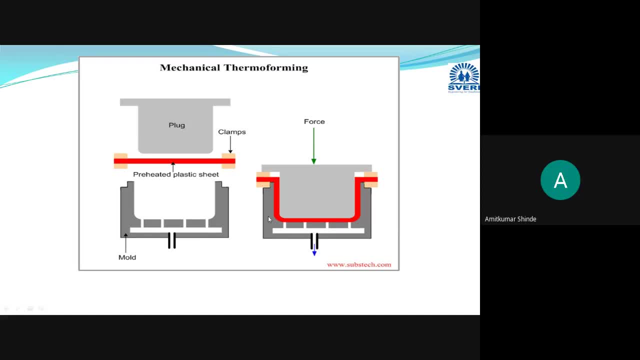 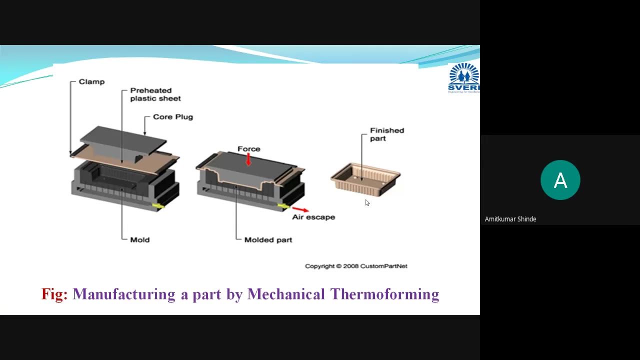 with the final product by releasing this mold and you have to release this plunger or punch also to get the final product. the same stages have explained with the help of for that same product. okay, you can use any preparable method to apply the force. it is not compulsory to go for vacuum. 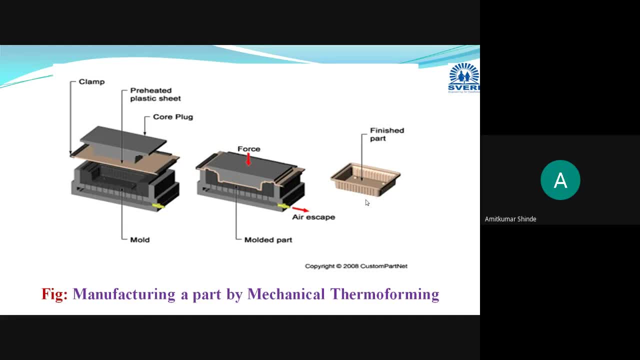 thermoforming. or you can say that pressure thermoforming or mechanical thermoforming, according to your means, economics of your processes, you can choose it. okay, now, in this same stages, are there. this is your mold. or you can say that the mold cavity is there in this clamp, the thermoplastic sheet is. 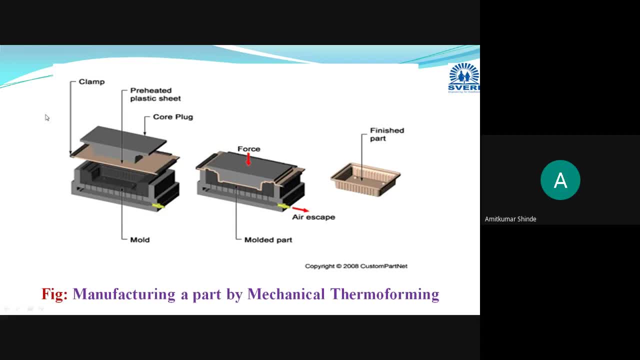 first you have to collect it and you have to hold it and it is heated with the help of some heaters and with the help of one plug- or you can say that punch or plunger- the pressure is applied in downward direction and due to heating already it is soft in nature. then it is pressed against the 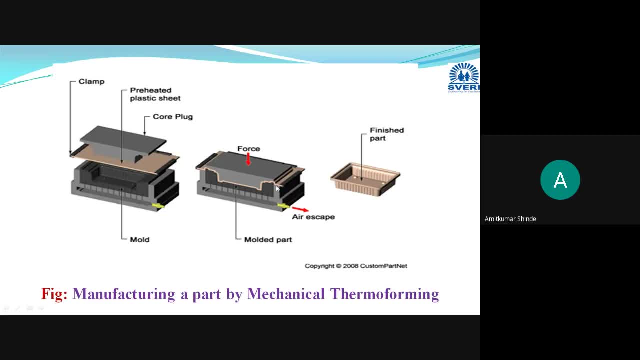 mold walls to acquire the desired shape, after sufficient amount of cooling from the final product is obtained by removing the plunger and this mold. okay, and here one at the bottom side from the outlet is provided so that air can escape from that mold. okay, when you apply. 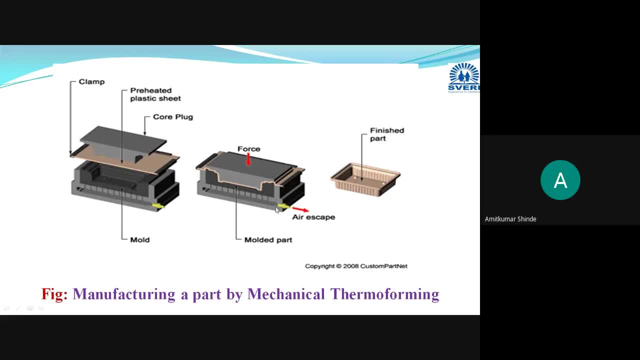 the sudden force, some air may be there and that air make it will get escape, or a way to escape from this outlet. okay, this is air escape. in this way, the final product is obtained with the help of this mechanical thermoforming. so in this way i have explained this on all three types of the thermoforming processes. 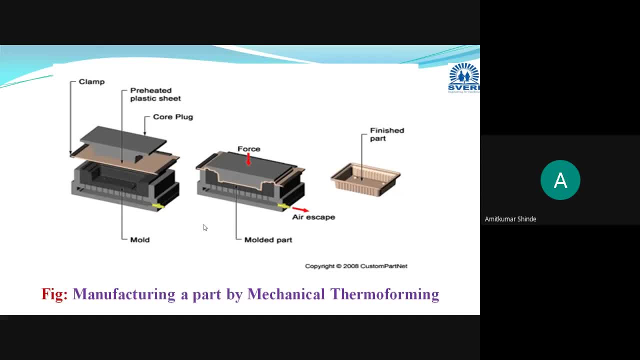 under pressure, natural oldest chiseling bowl, any lock at the same time. just pump down a little bit. i will mostly bring you praising all the three types of the thermal form processes. let me show that. okay, because this panel is fit in, the bottom priest is held likes toれ. 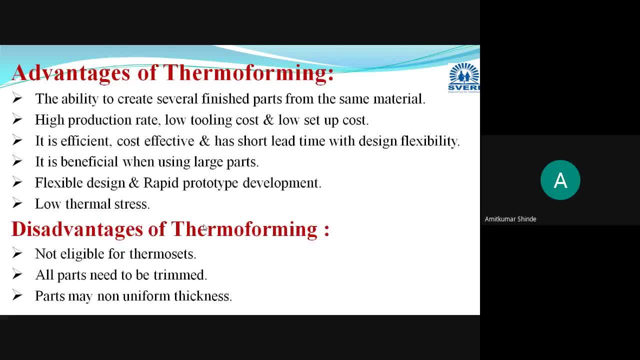 and then we will move towards system. before application part we will check the some advantages and disadvantages of thermo forming process. the first advantage is: okay for the same kind of material. okay form, same kind of material as it is available in the form of sheet. you can give the different kinds of. 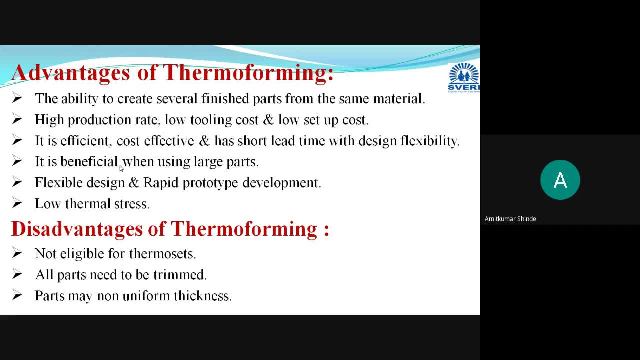 shape. okay, different shapes can be given to the same material. that is the first advantage. then here the rate of production is very high and whichever tooling cost and setup cost is there, it is very less in this thermo forming. that is the second advantage: high production rate with less tooling cost and a less 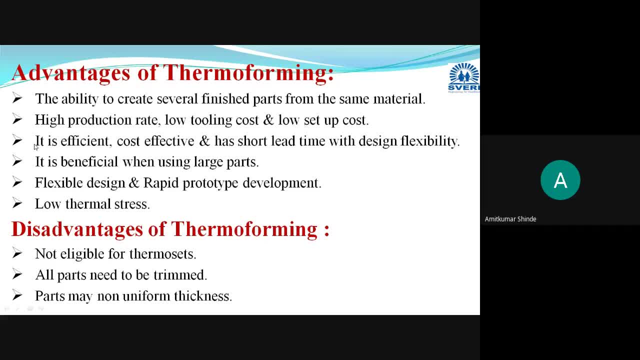 setup cost. okay, the same is explained here. it is a efficient process because it is a cost-effective. why it is cost-effective? cost of tooling is less and setup cost is very less and short lead time. shortly time means the whole process. it will start from collecting the sheet, plastic sheet- to get the end product. it can be. 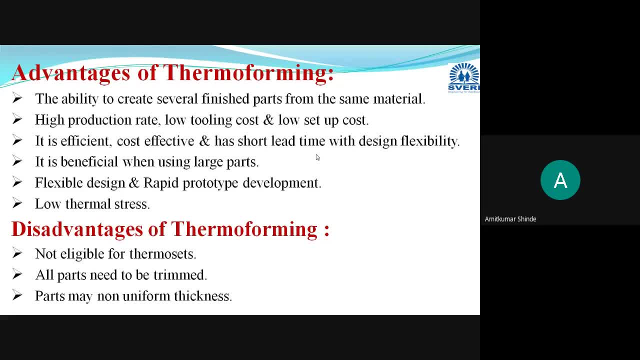 done with the shortest time possible time. okay, that's why it is termed the short lead time and due to the short lead time here we can give any kind of the shape and size. okay, by changing the- you can say that your mold design- you can change the shape of the. 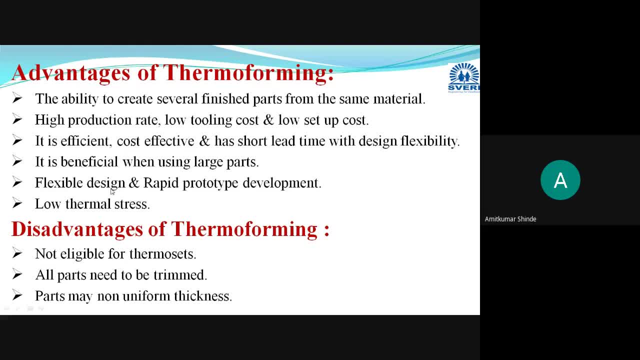 product, then you can do this, apply this process to open larger sized products also. okay, some flexible designs. so whenever you are making a prototype material, any kind of component, before manufacturing it, actually some prototype is made, okay, exact replic of the final product that is made with the help of this thermo forming process only, and as here we are performing. 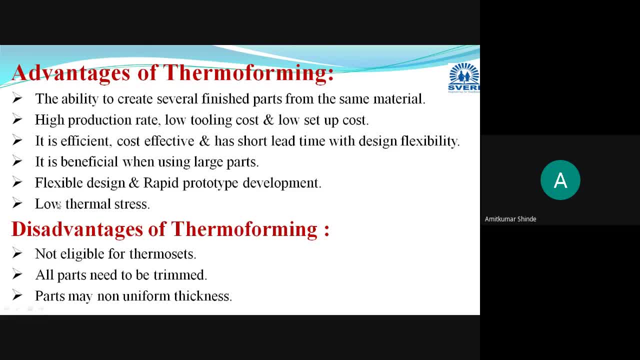 some sheeting operation and then we are applying the pressure. thermal stresses will be very less. okay, temperature range is not so high. some it is below 200 degree Celsius and after that, first we are it and after that we are applying the force. okay, due to that, thermal stresses. 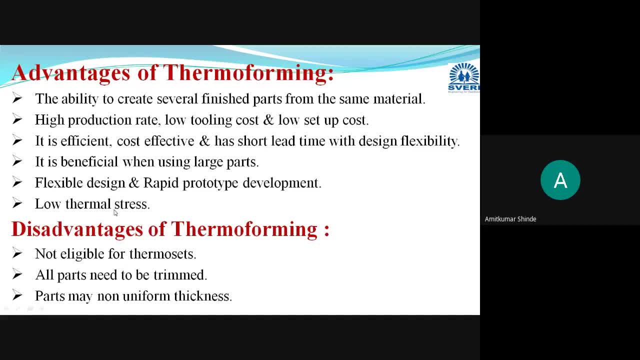 are very less. so these are some advantages. okay, I'll put it: you will get means from same product, different shape. the products of having different shapes and size can be obtained from the same material and it is efficient because it's cost of tooling and setup cost is very less and high production rates can. 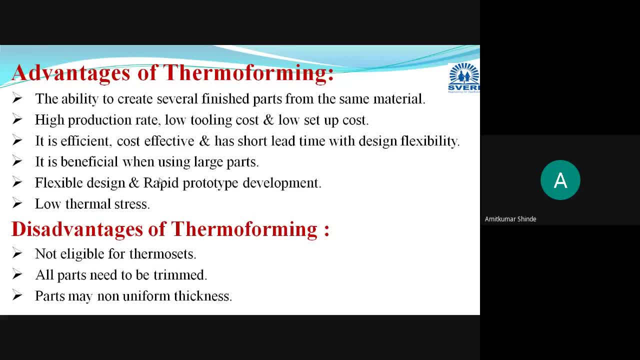 be obtained. it's lead time is very less or short. lead time, when we can be a manufacturer means design flexibility. is there different: small shape- the components or parts- and large shape- the parts can be manufactured and the thermal stresses are very low. as we are performing before applying the force, we 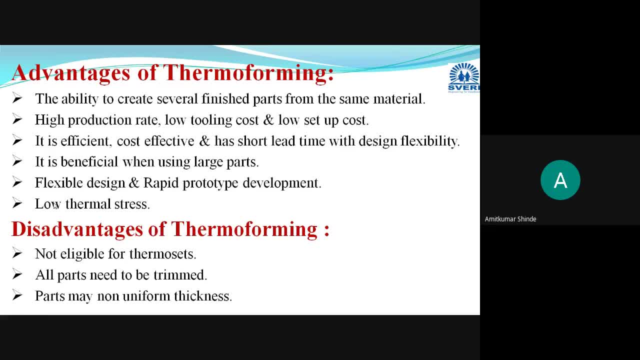 are performing some preheating or heating operation. that's why thermal stresses are very less. the advantage is of this thermoform and process. then what are the disadvantages of this process? ok, the first disadvantage is related to the use of material. this process is only useful for thermoplastic materials. we cannot. 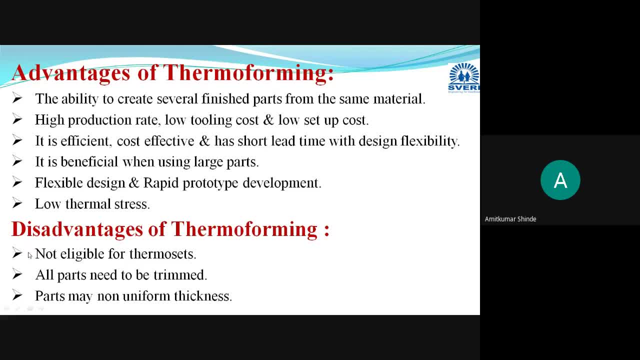 use it for thermo setting materials. we cannot use it for thermosetting material as the thermosetting materials cannot be rolled. or you can say that we cannot perform the calendering on some thermosetting materials. that's why, as sheet is not available, you cannot give the desired shape and size. okay, if it is. 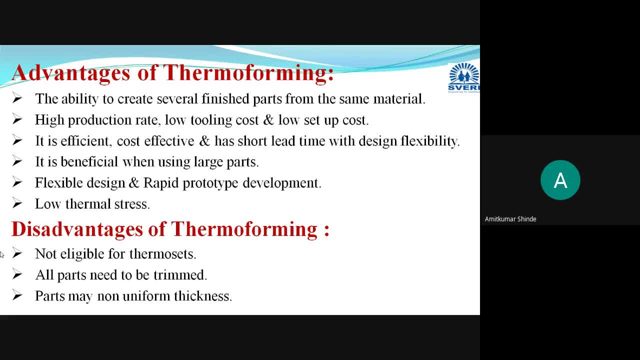 sometimes you may end up with the sheet, but the thermosetting materials cannot be reprocessed, remolded or reshaped. that's why it is that these materials are not suitable or eligible for thermoforming operation. okay, not eligible for thermosets or thermosetting plastic materials, then. 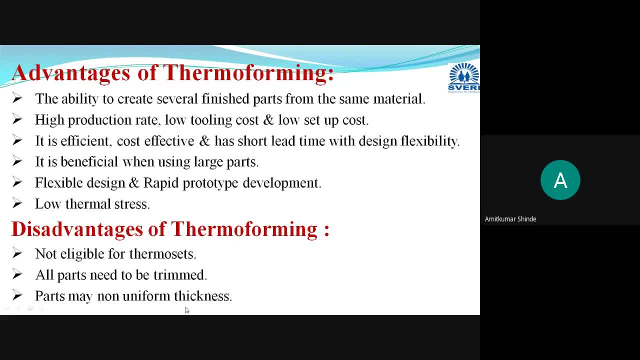 sometimes. sometimes the parts may not be uniform throughout. whichever thickness is there, uniform thickness may not be obtained. uniform thickness may not be obtained. and another disadvantage is: all parts manufactured require some trimming operation. some extra material may get attached to the final finished product. that's why you have to perform some trimming or small machining. 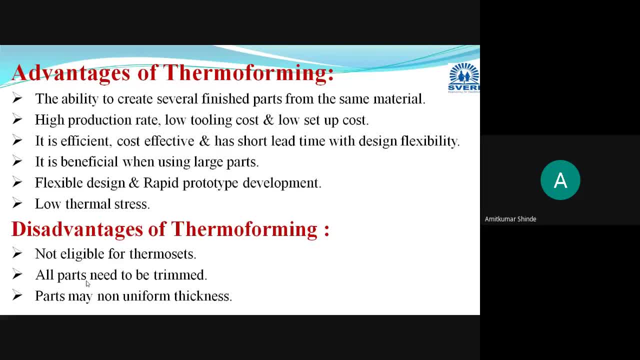 operation too. remove that extra material from your finished product. so these are the disadvantages of thermoforming processes. it's not eligible means this process is not eligible for thermosetting materials. then all parts required trimming or slight machining operations, and parts sometimes may not have uniform thickness. okay, these are the disadvantages. now these are the some applications. 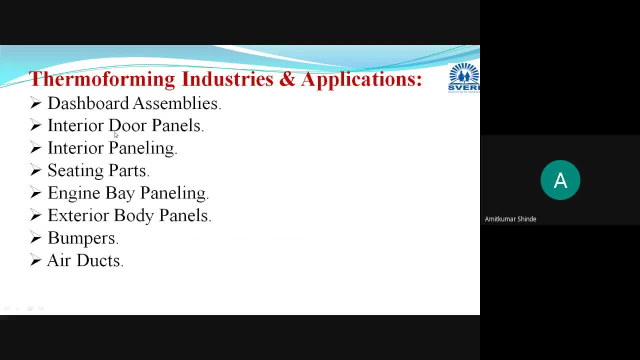 some dashboard assemblies, interior door panels, interior panelings- okay. these components generally are used in your automobile sector. okay, in the automobile sector, or some components, you can use it in the your home decoration also. okay, whichever bumpers are there, air ducts, exterior body panels- you can say that. 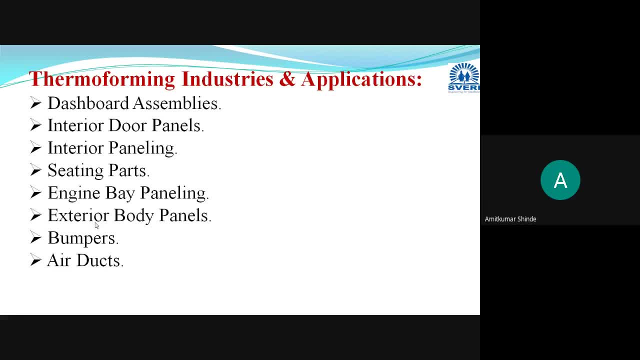 that bumpers are there, exterior bumpers or exterior body parts, or you of your are two four wheelers, okay, four wheelers, or your two wheelers, some sitting parts of your four wheelers or two wheelers, these all are manufactured from this. thermoforming operations only, okay. 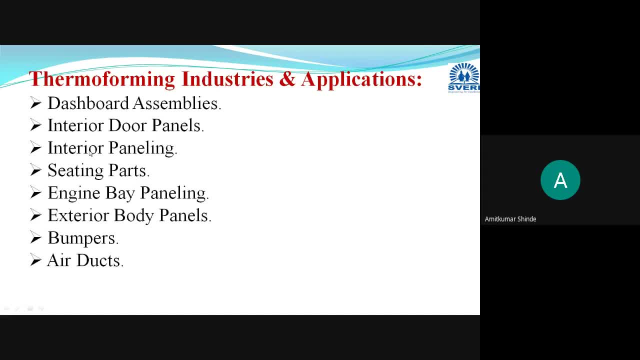 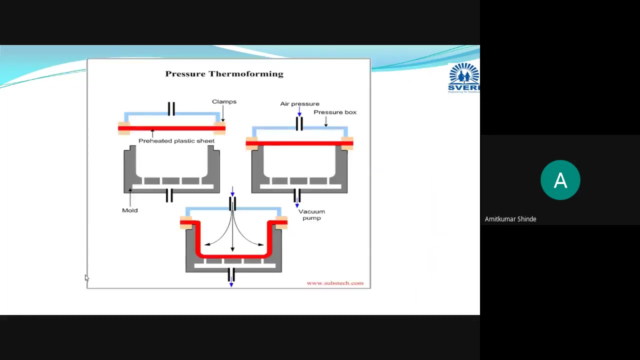 dashboard assemblies, interior door panels, then exterior door panels, also sitting parts, then bumpers and air ducts. all these components are manufactured with the help of this thermoforming process. only okay. so in this way we have completed this thermoforming process with its basic concept, basic principle and its three types that we have covered: pressure thermoforming, vacuum thermoforming. 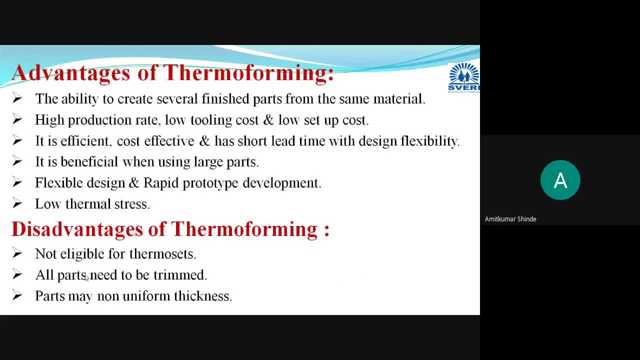 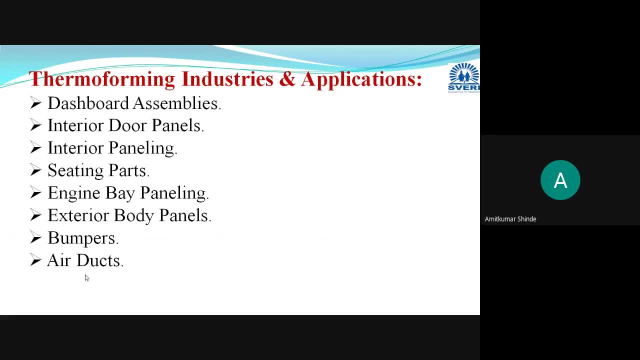 mechanical thermoforming, then we have discussed some advantages, disadvantages of this thermoforming process, along with its applications. okay, in this way this is the second chapter is already completed. this is i have taken just for your information purpose. sometimes they may ask a basic question related to this thermoforming. 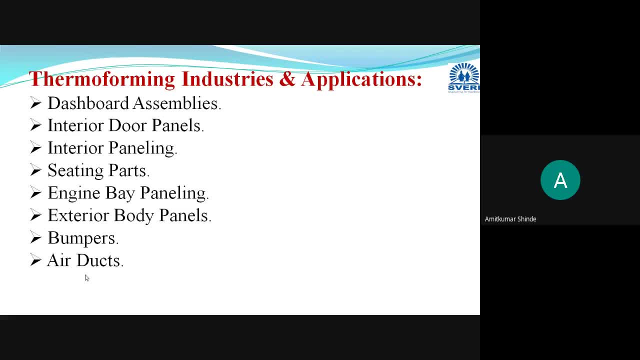 concept also, so that you just go through it. small stages and types are there, depending on the mediums, you can write it. some advantages, disadvantages and applications you have to write okay. so after this we will move towards. now i will solve some mcq questions from your booklet, okay, and i will instruct you to solve the second test which i have provided. 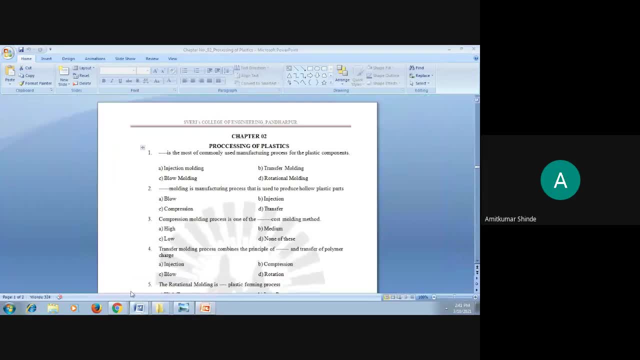 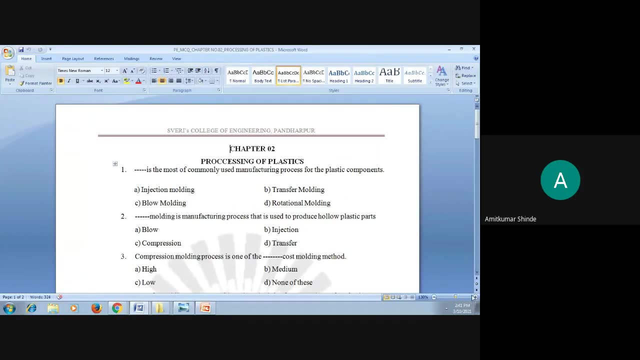 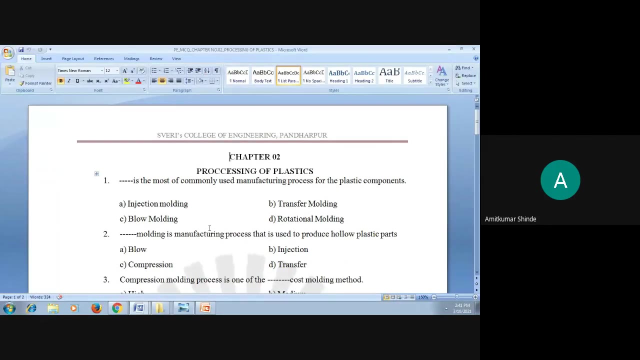 okay, okay now here these are the msecurity questions. okay, now i will read it and you you can give me answers by entering in the chat box. okay, the first question is like this: uh, which process- okay, out of this following- is the most commonly used for manufacturing of the plastic components? 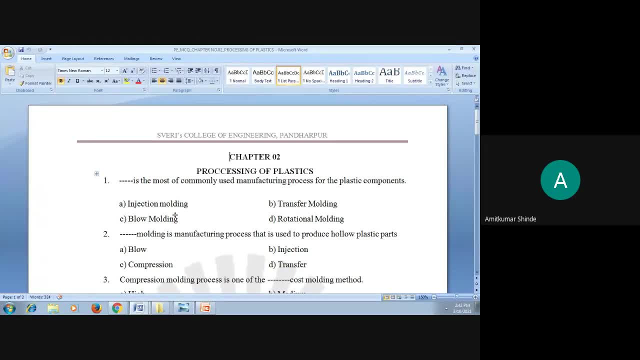 okay, most widely used the process for manufacturing of the plastic components. if you are having the knowing the answer, you can enter that in the chat box. okay, I will provide you the answer. the injection molding process. it is the most widely used in the manufacturing of process for the plastic component. even 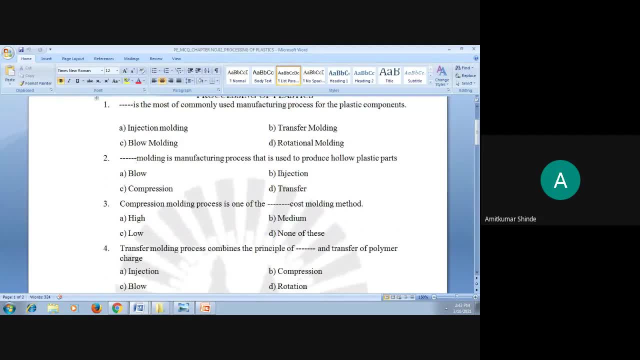 second question: okay, out of these four molding processes, which molding process? okay, it's used to produce hollow plastic parts- blow molding, injection molding, compression molding and transfer molding. out of these four molding processes, which method is used for? okay is the correct answer. blow molding is used. a blow molding. 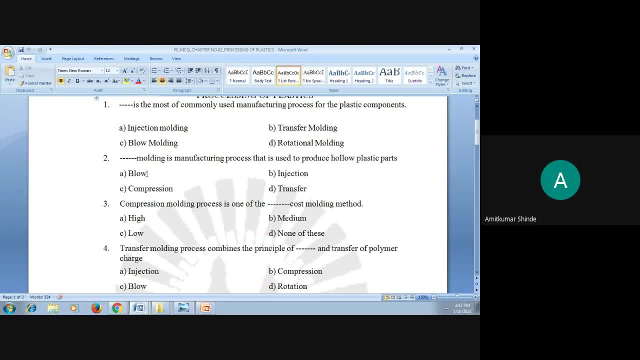 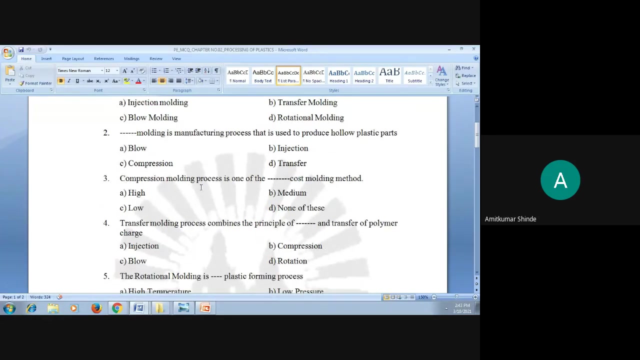 different water bottles are manufactured with the help of this. okay, sometimes there may be another option like rotational molding. okay, if blow and rotational, both options are there, then your answer will be a and B. okay in multiple choice questions. then third question: compression molding process is one of the 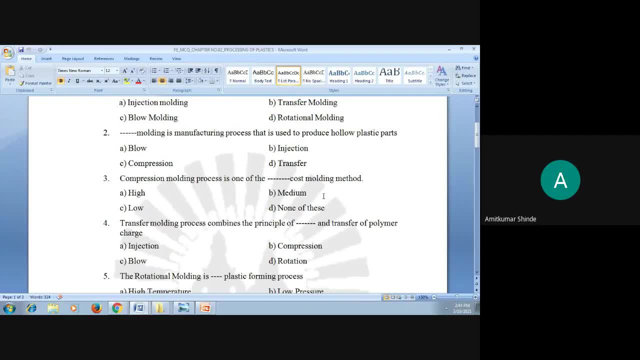 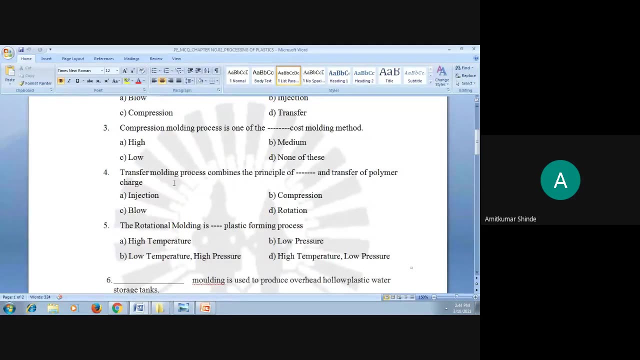 means whether it is a high cost or medium cost or low cost for molding method and this is a high cost molding method. okay, in this advantage of this compression molding process. you can get that answer in question number four here. transfer molding process combines the principle of estas adi and transfer of polymer charge. okay, transfer in the transfer. 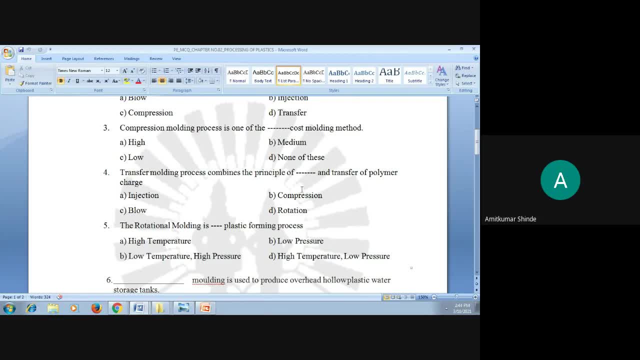 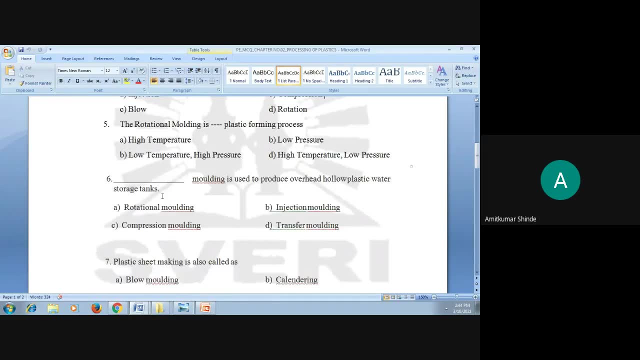 molding process is nothing but the polymer charge is taken in one transfer pot and then we are compressing. it means compression. answer is the compression. the rotational molding process is a dash-dash. you can say, than the plastic forming process already. areneg聯, etzt is nas dash. you can say that the plastic forming process already. as I said, media. we use? we use lumik 엄마, 2 umm, ummm. natural molding process is comenач Vacuumِّ reduction do creating the mineral формjan capçal chapel across on the bed. 그러니까, now I sharpening, we are going to, gibt es the superst diarrhea of, of storing the material to compare, of comp plugging지 to leave the processIF you can verify if poly 이번ally transform movies are applied, any change in any other way except an没有. 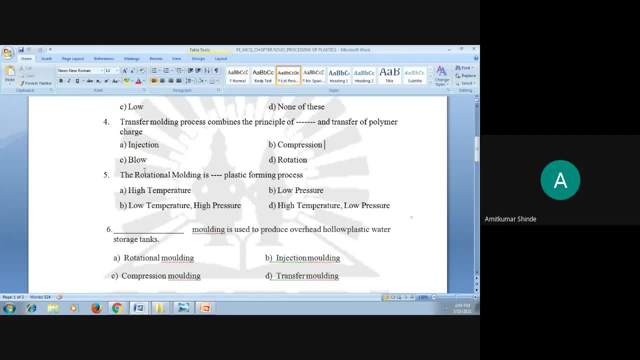 Already. I have discussed this while taking the session on this rotational molding. Rotational molding is a high temperature, low pressure forming process. Answer is 4.. D, That is a high temperature. In the rotational molding, temperature is high and pressure is low. 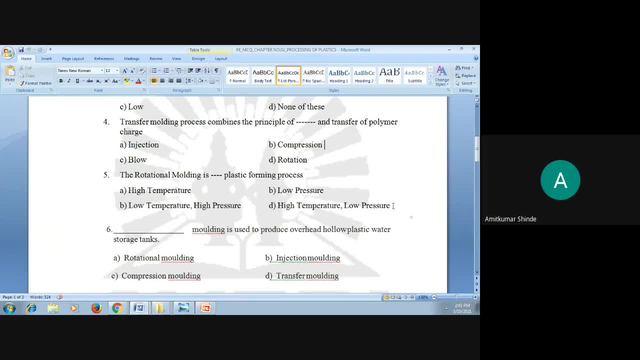 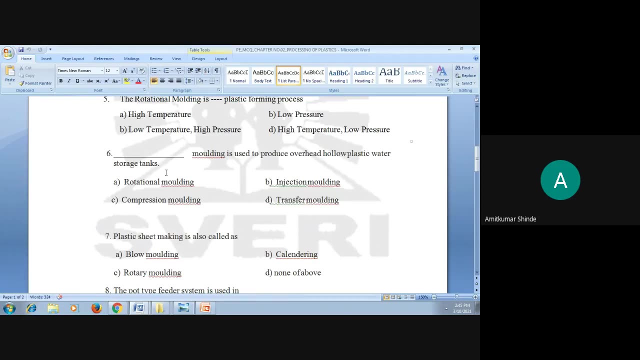 We are heating that powder and we are rotating it By. actually, we are rotating it. Answer is high temperature and low pressure. Now, with the help of which process holoplastic water storage tanks are manufactured? That storage tanks are manufactured? with the help of which process? You can provide an answer in chat box. Its answer is rotation. 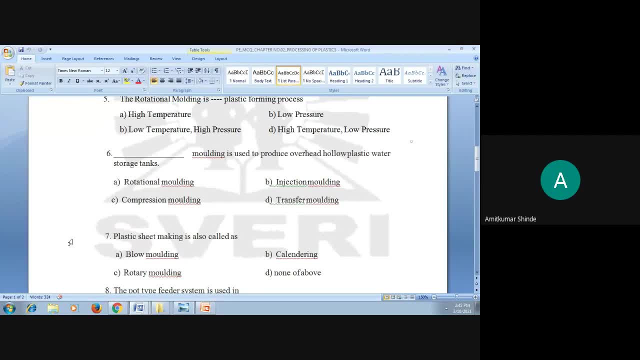 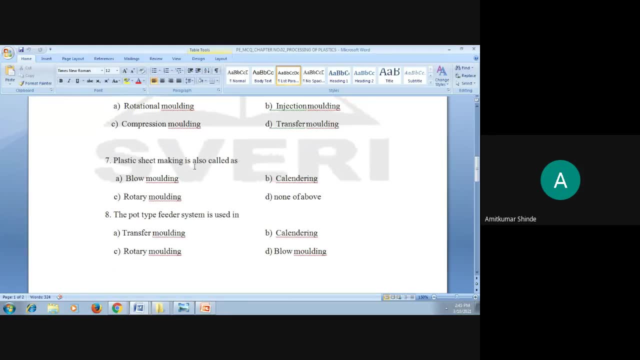 Rotational molding Storage tanks. Water storage tanks are manufactured with the help of rotational molding. Then plastic sheet making process is termed as calendar. Then what type feeder system is used? in What type feeder system means We are collecting the charge in the one transfer pot and it is then placed in a mold cavity. This is in transfer molding process. 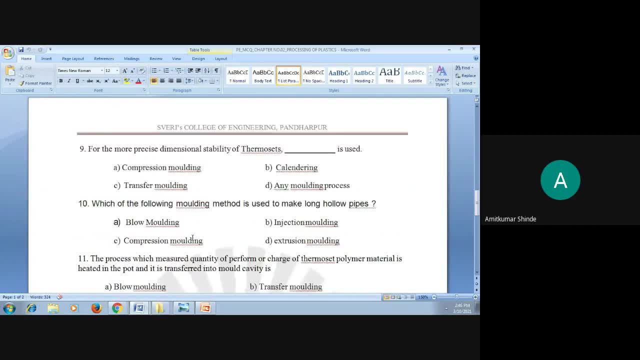 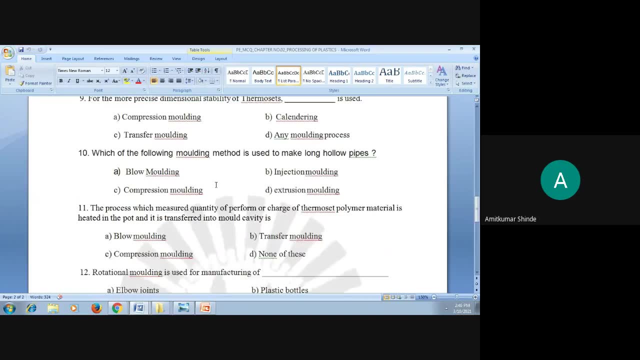 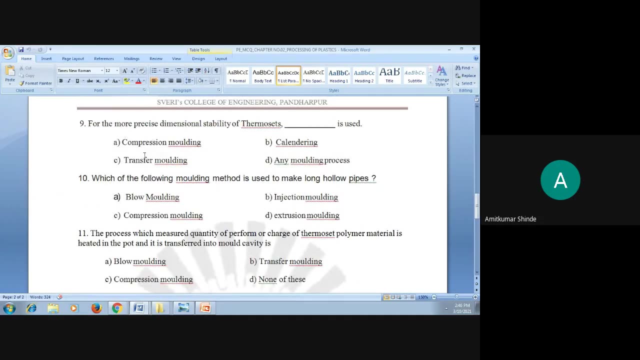 This is in transfer molding process. Well then, the last four questions are there. Here are some three. four questions are there. Well, for the next stage, this is related to the thermal fitting material to get the precise dimensional ability. Now for Thermo-setting materials, some more processes are used. 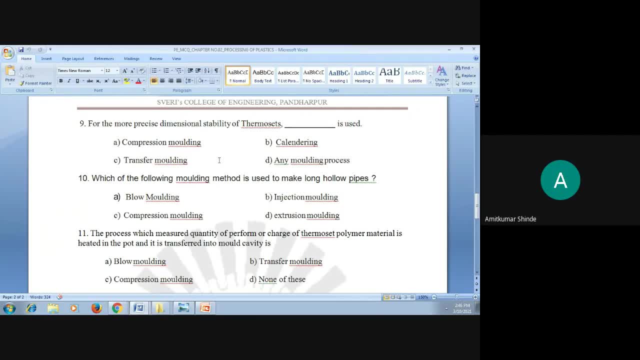 Ok, OK, Yes, Ok, Yes, Yes, Yes, Yes, Yes, Yes, Yes, compression, transfer and rotational can also be used here. this calendaring we are only performing means it is giving in the shape of sheet and this is on. 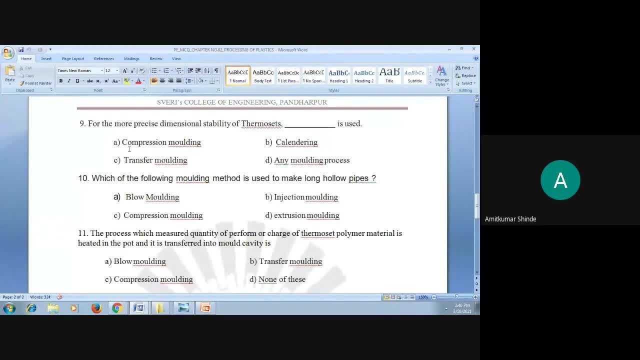 thermoplastic material only. and then, out of these two correct answer will be transfer molding. okay, because in compression molding we are directly applying the pressure and here we are collecting charge in one separate pot and it is then transferred in the mold cavity. that's why the desired 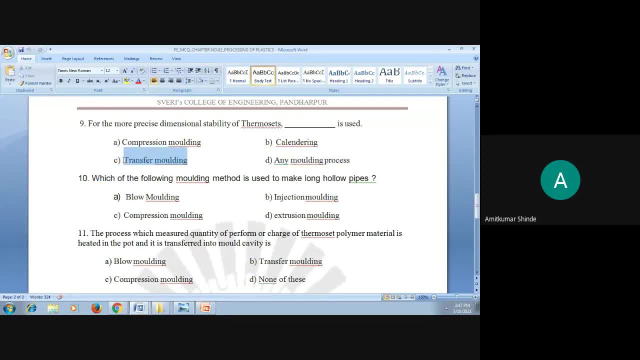 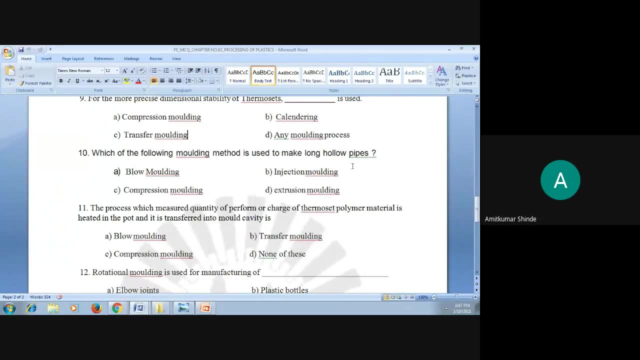 dimensional accuracy is more in the transfer molding. compression, holding, transfer molding will provide you better dimensional stability accuracy, then, which of the following molding is used for making long hollow pipes? that PVC pipes, whichever PVC pipes are there. or you were that irrigation pipe for that drip system? okay, drip system in your agriculture. that pipes are used. 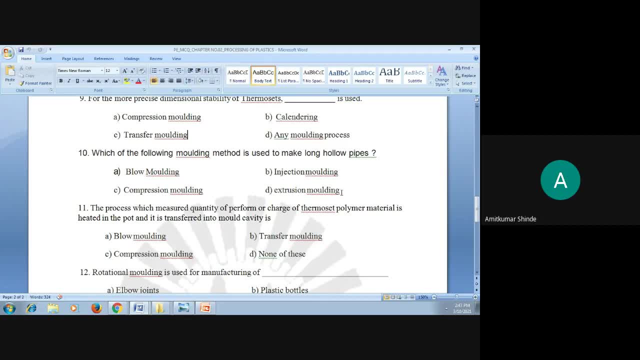 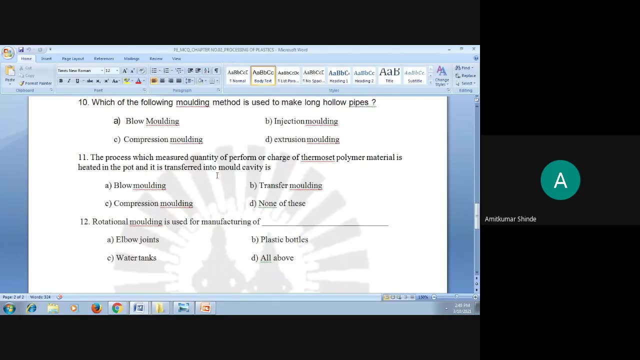 that all pipes are manufactured by the extrusion molding process. okay, extrusion molding process. hollow pipes will be manufactured with the help of this extrusion molding. okay, then this process: such a measured quantity of preform, a charge of a thermostatic polymer material, is heated in the pot and it is transferred in the mold cavity. okay, heated. 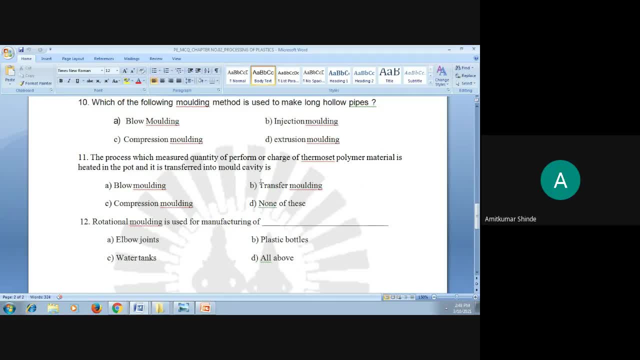 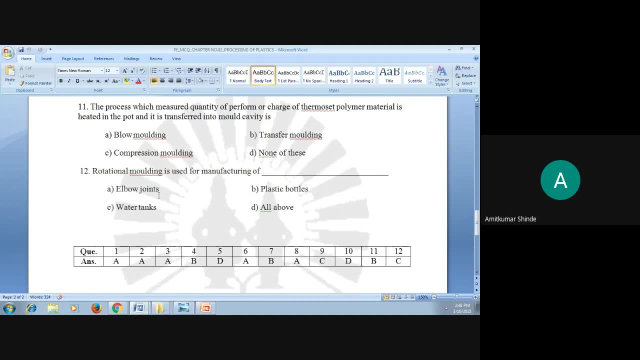 in the pot and transferred. it is done in transfer molding. answer is B. and the last question is: rotational molding process is used for manufacturing of? is elbow joints? this is not the correct answer: these elbow joints and these plastic bottles only. the correct answer is: water tanks are manufactured with the 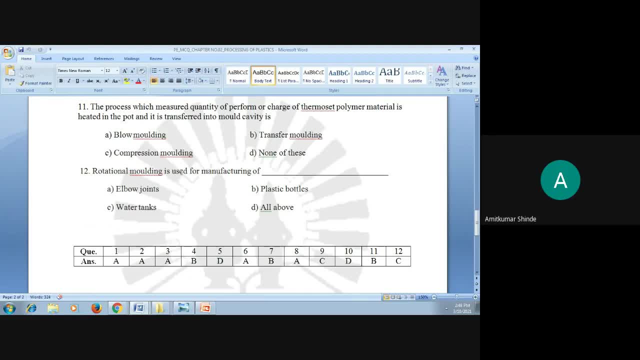 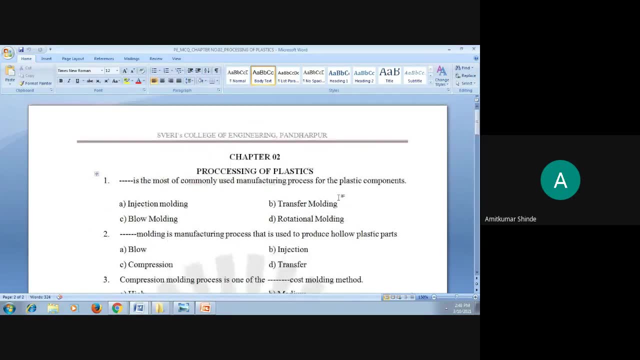 help of the rotational molding process. okay, for all questions. you know I'm sure I have provided here this sheet. I will upload on the study material sheet, chapter wise also. initially I have uploaded all the MCQ questions in one sheet. when I will finish each chapter after that I will upload this sheet in. 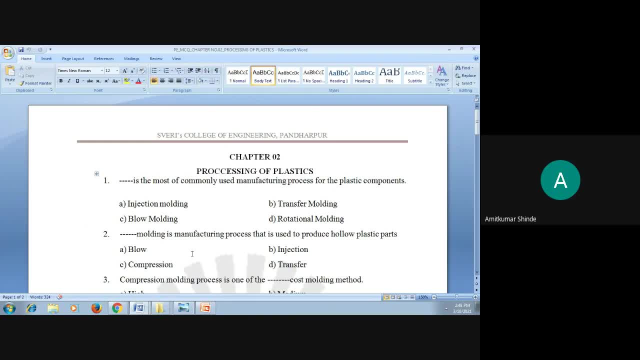 this study material sheet. okay, in this way, our first two chapters are already completed and I already have sent you the MCQ test. please attend the MCQ test for the second chapter. it will get closed after two hours. okay, it will just require 20-30 minutes, or. 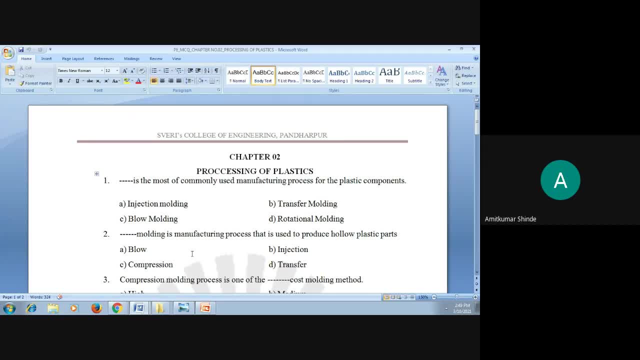 if you do it in fast way, you can finish it in 5 or 10 minutes also. okay, only 10 questions are there. it solve it now. in this way, we have completed this chapter. okay, now I will summarize this chapter, what we have studied in this. 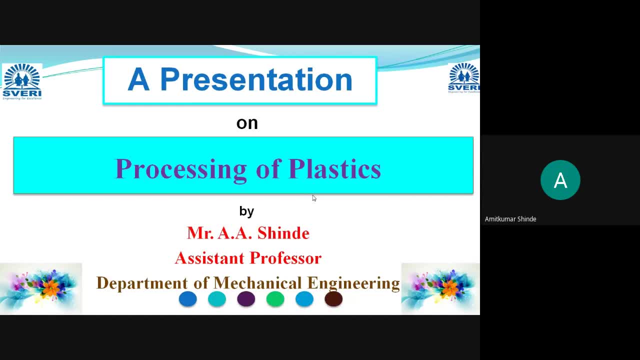 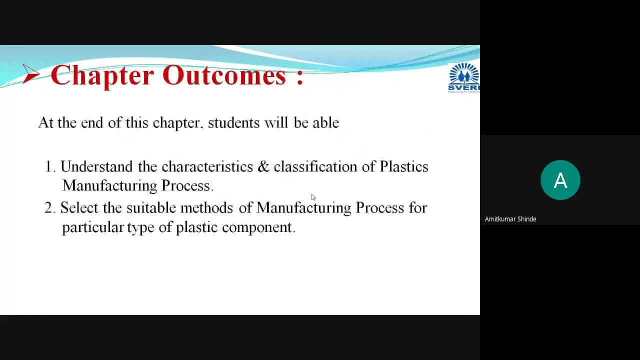 chapter in this chapter this is the processing of plastic难以约 speaking processings of plastic難以约. employees of plastic be moved directly from Tortoise to the home object, so a single chamber making took months before application of plastic выпол. in this we have started with the prerequisites title of the chapter, the 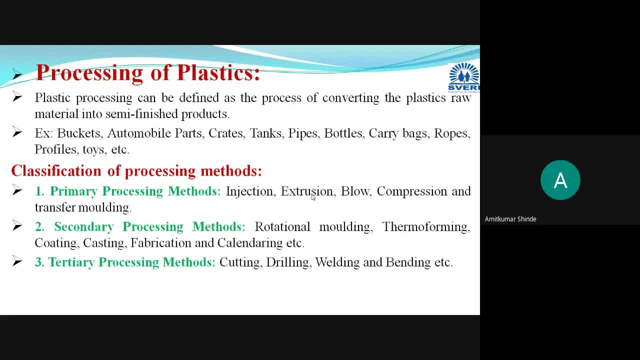 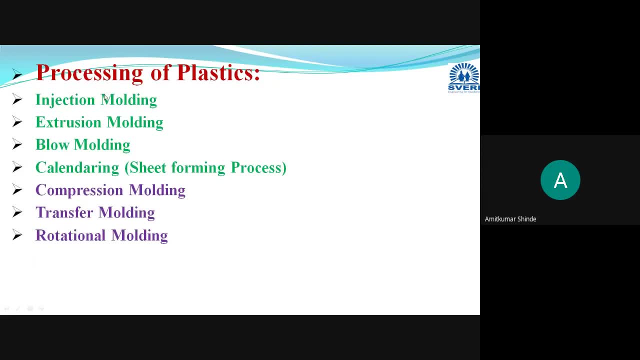 first we learned processing of plastic and its basic classification. then which methods, processing methods are used for thermoplastic materials: injection molding, extrusion molding, blow molding and calendaring. these are used for thermoplastic materials and compression molding, transfer molding and rotational molding. these three methods are generally is for thermosetting materials. 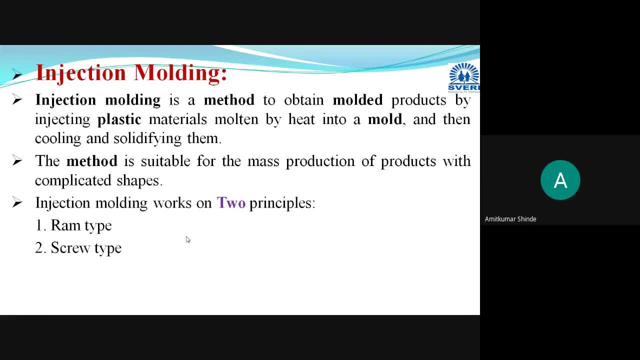 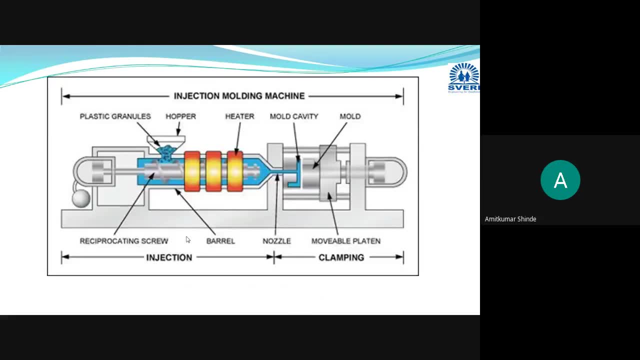 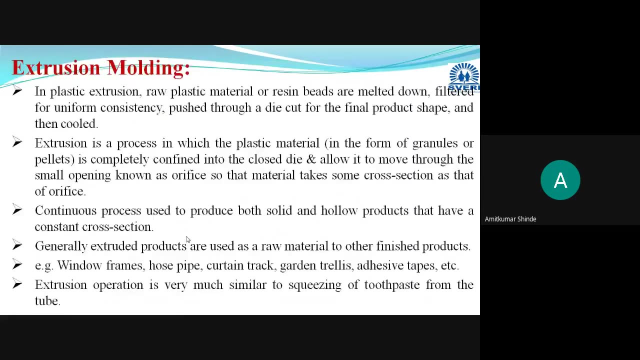 then we have seen discuss the concept of injection molding, along with its basic principles. is types, this basic principle then, its types, advantages, disadvantages in some applications. next we have discussed the extrusion welding, how different kinds of different PVC, hollow PVC pipes manufactured along. first we have learned the concept of extrusion molding, along. 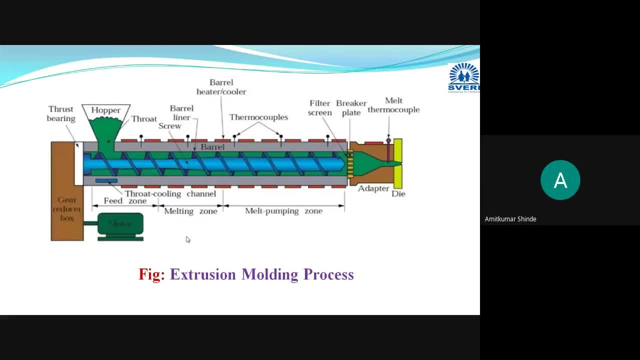 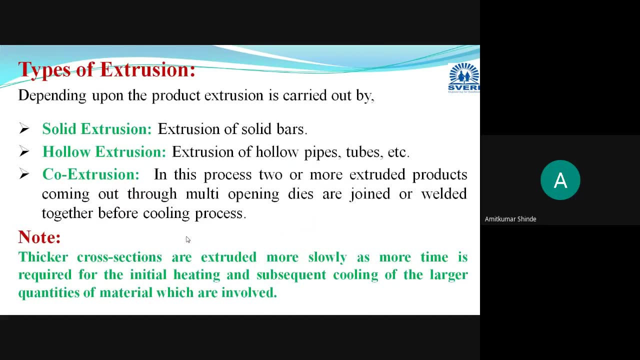 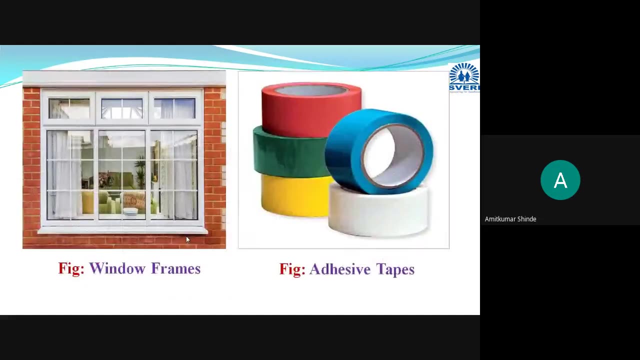 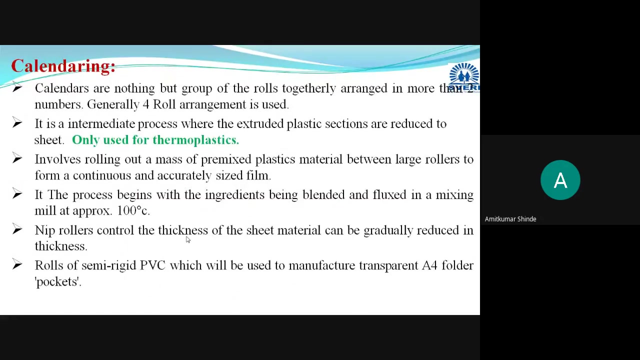 with these steps involved in it. okay, this is the extrusion molding. two types of the extruders, types of the extrusion process, applications: okay, hollow pipes, adhesive tapes, all these can be manufactured at one day, as this advantages. then after that we have done the calendaring process. 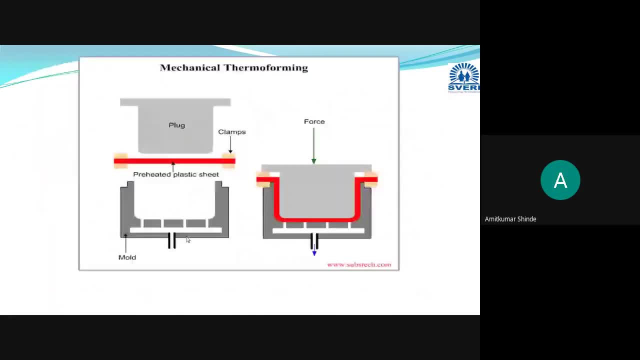 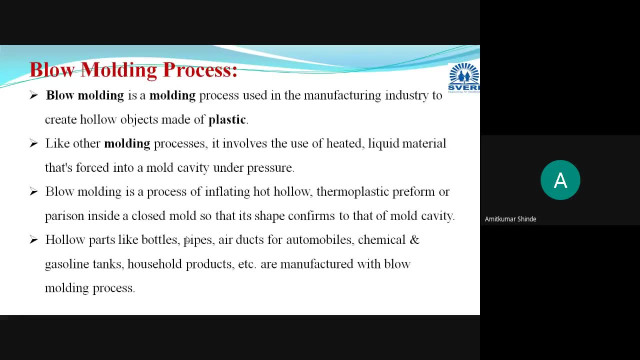 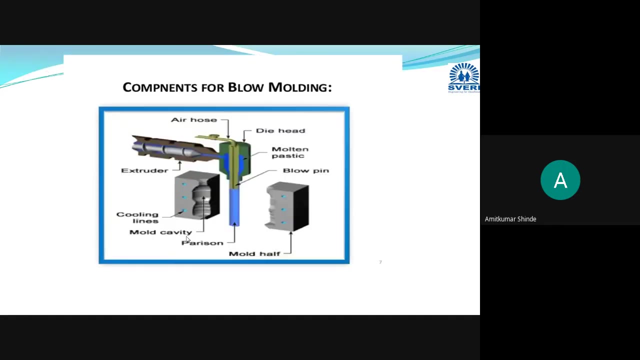 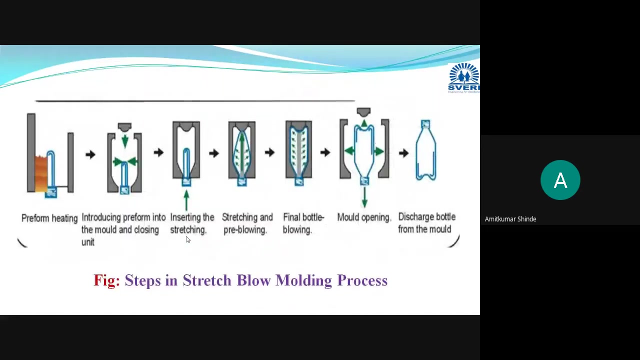 okay, and then this thermal forming- just now we have finished it, okay, and blow molding process we have means this: with the help of this blow molding process, we can manufacture deep, hollow plastic bottles, hollow pipes, different. okay, this is the concept of blow molding process, basically concept states, classification and then how it's: different types: injection, blow molding. 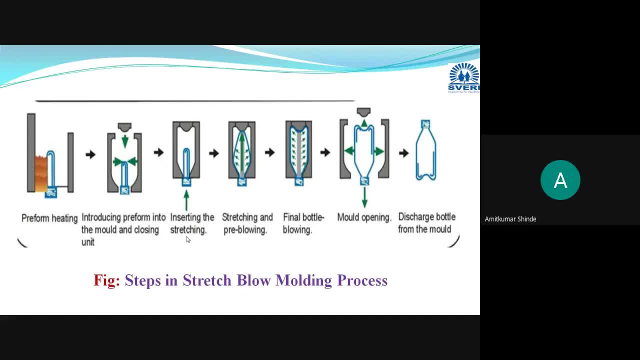 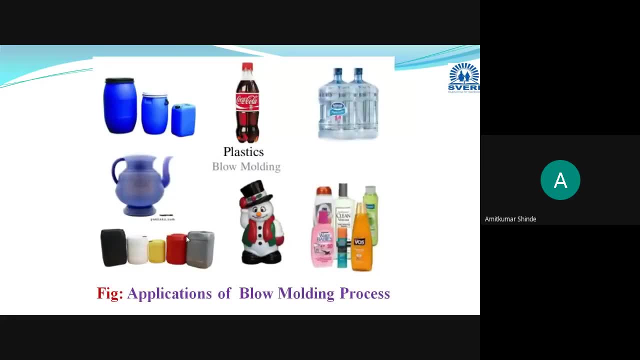 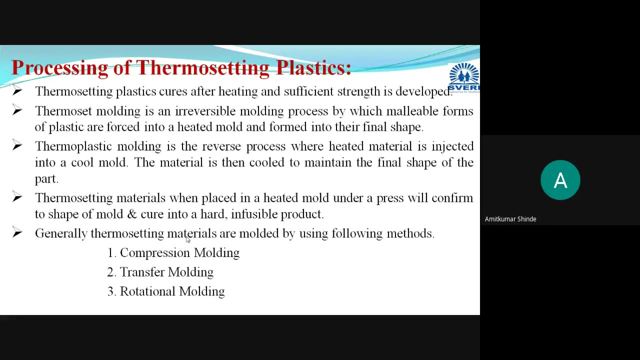 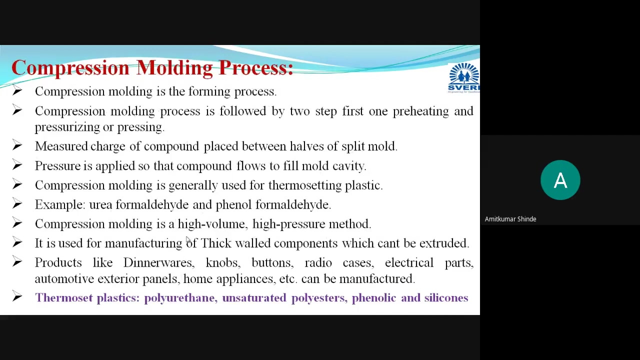 process- extrusion, blow molding process and stretch blow molding process- and different materials and different components means its applications, along with advantages, disadvantages. we have discussed this. then, after that we have discussed this thermo setting materials, processing of thermosetting materials, materials, and that we have first learned the compression molding process. 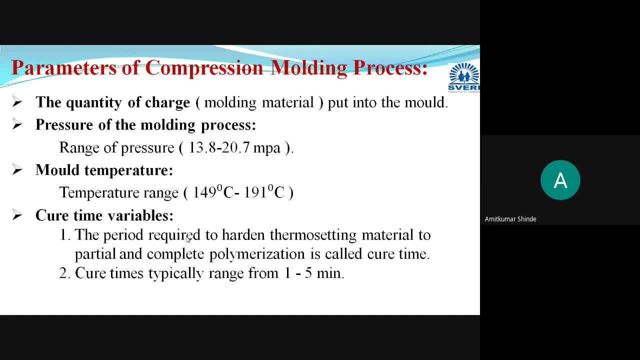 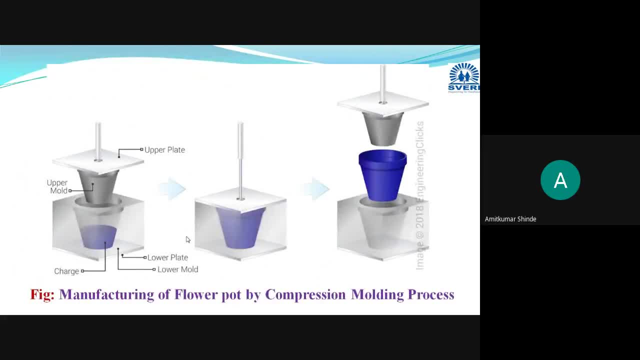 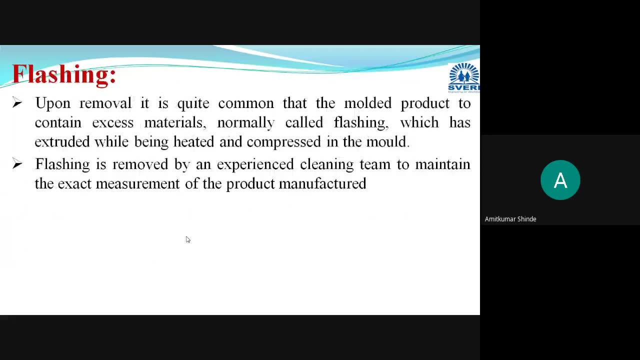 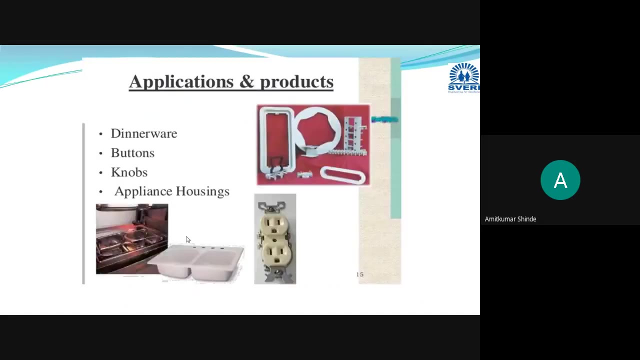 with its basic working principle and parameters. this is working principle. one practical example: manufacturing of the flower pot by the compression molding process. then advantages, disadvantages, some disadvantages: how- what is the meaning of flashing, how it is removed? and applications of compression molding process. then transfer: molding process: its working principle. 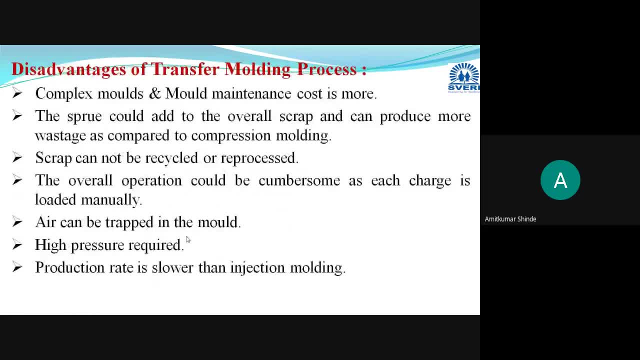 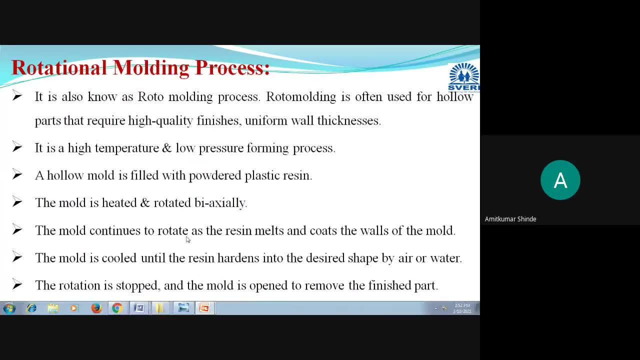 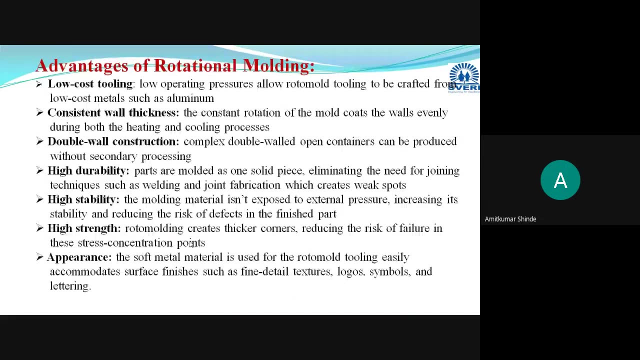 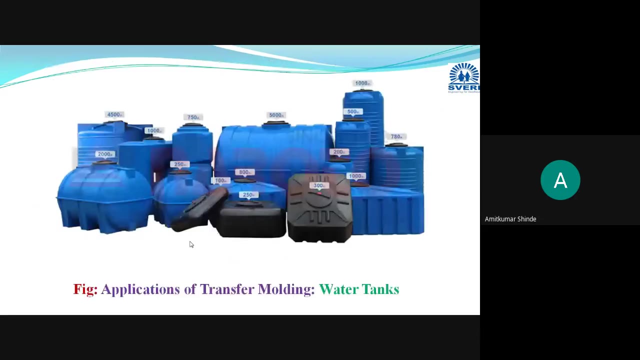 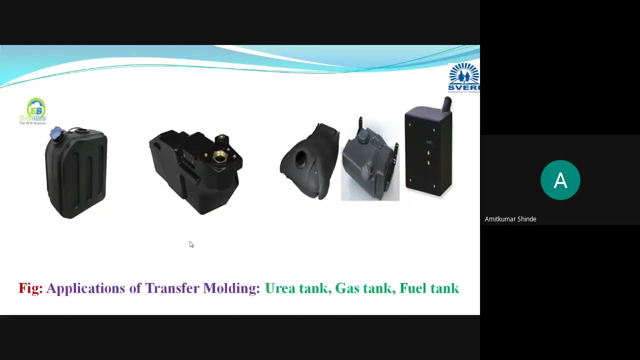 multi-carriage transfer molding process in its advantages, disadvantages, different applications we have learned here and the rotational molding process. tapes involved in the rotational molding process. advantages of professional molding process, so that disadvantages of rotational holding process and some applications like water tanks, military utility boxes and different urea tank gas tank. 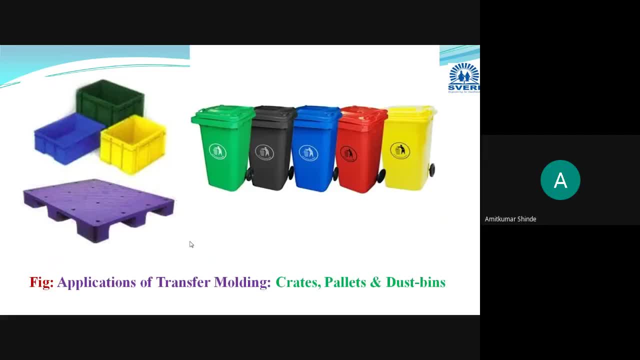 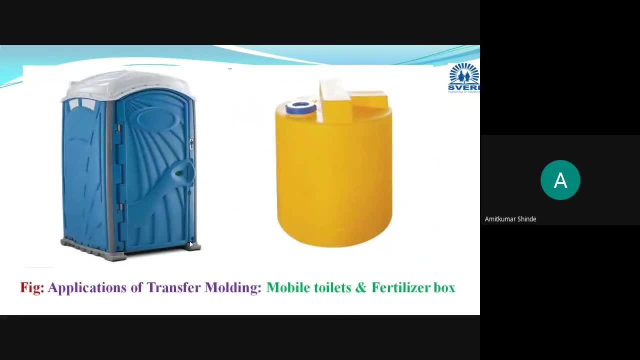 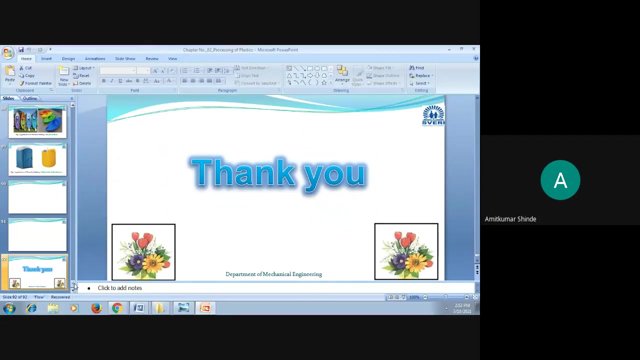 fuel tanks, road barrier, children slides, crates, pallets, different dust beans. then your kayaks, boats, mobile toilets, fertilizer box. okay, all these are manufactured from that rotational molding process. in this way, we have completed this. okay, processing of the plastics. please attend the mcq test today, only within the next two hours. after that, it will get closed. 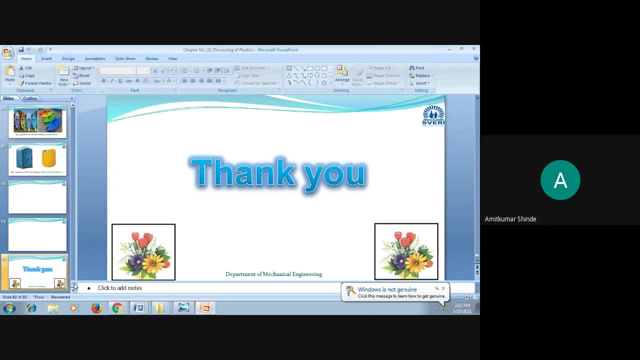 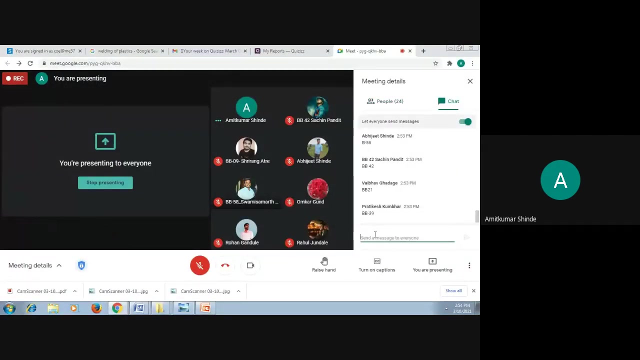 and those who have joined. you can put that- your attendance- in the chat box. thank you for attending this session. from next session, i will start the welding of the plastics. okay, welding of plastics. okay, so we have discussed the mcq questions with the answers. okay, thank you for attending the session. you can continue with your remaining sessions, thank you.